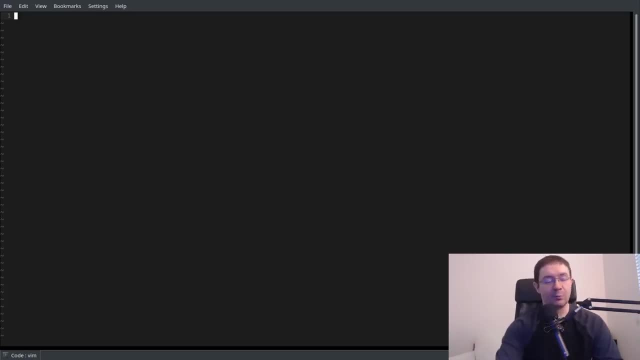 All that said, let's go ahead and get started. We begin with our imports. We are going to need the base torch package as t torchnn to handle our layers In this case, since the lunar lander environment is just a simple eight vector, eight element vector observation. 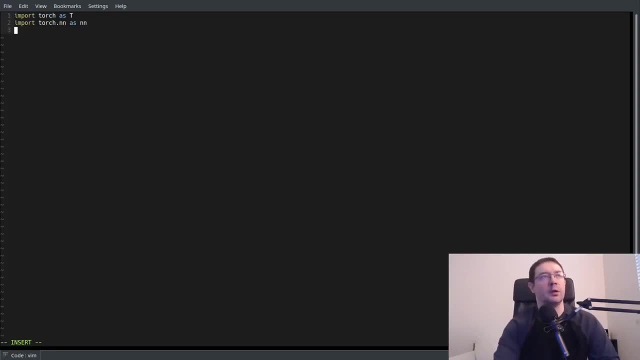 we're only going to use linear layers, We're not going to be needing any convolutional layers And we'll need nnfunctional for the ReLU activation function for our deep neural network And, of course, Optum for our atom optimizer. and we need NumPy to do various NumPy type things. 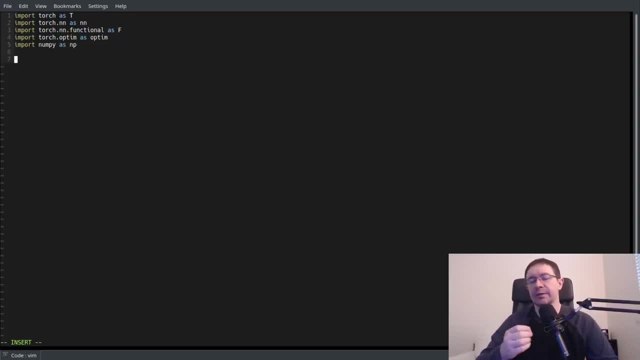 So we're going to use a reduced kind of a reduced solution from my course. In my course I break everything into highly modular chunks, everything. When you are in the DeepNurl area, you're going to have to use an int and an option. I'm going to 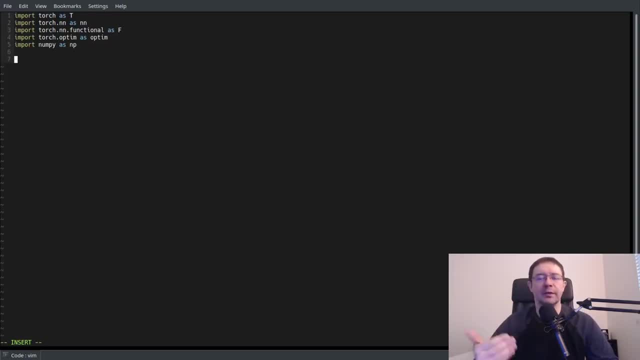 do my int first, so I know that this is a very simple way for you to know how to recycle Is kind of like a bunch of Legos you place together that you can mix and match between different projects Along with the command line interface. very clean solution here. 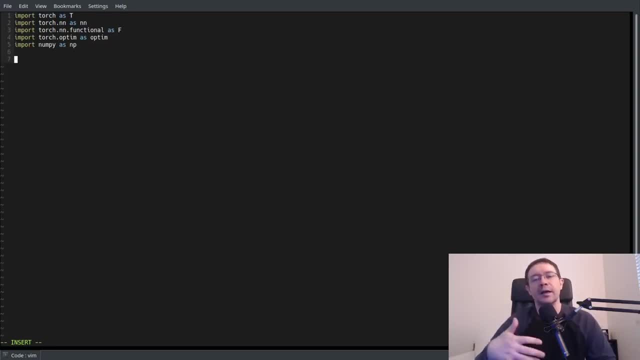 We're just kind of kind of stick stuff into two main classes and kind of mix up some functionality, Because it's just a YouTube video, But it's going to do more or less the same thing and our two classes are going to be the class for the deep Q network. 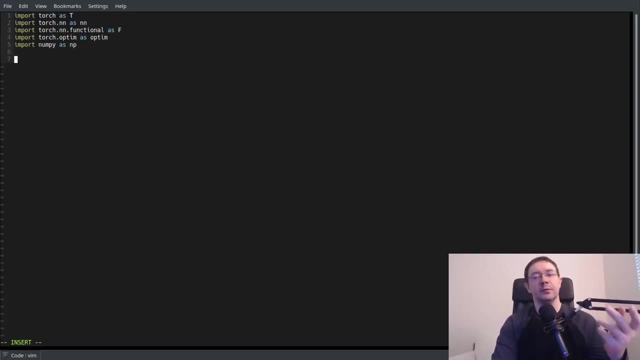 And the other class will be the class for the agent region. The reason behind this is that an agent is not a deep Q network. rather, an agent has a deep Q network. An agent also has a memory, a way of choosing actions as well as learning from its experience. 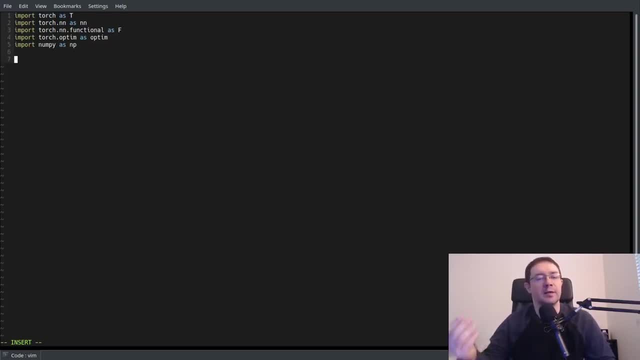 Whereas a deep Q network is precisely that, is just a neural network that takes a set of states as input, now puts the agents estimate of action values for each given state in the input. And if you are unfamiliar with PI, torch, the convention is that every class that extends the functionality of the base neural network layers 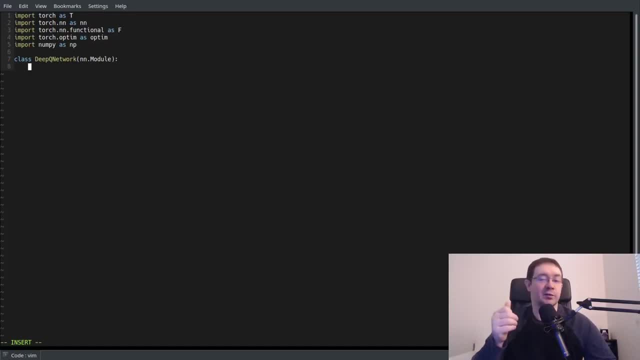 derives from an end up module. this gives you access to a number of goodies, in particular the Parameters to perform the optimization, as well as the back propagation function, so we don't have to write back propagation ourselves. This will take in a learning rate: input dims- FC. one dims, FC, two dims and and actions as 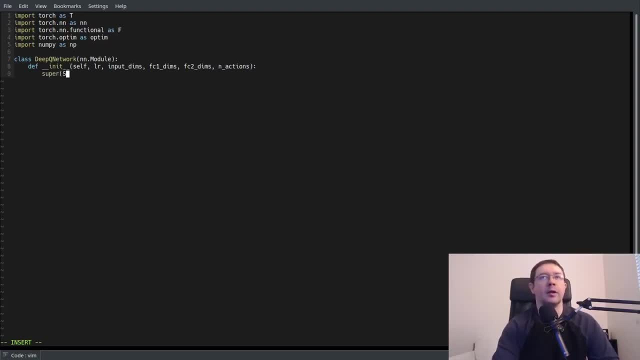 Input and you want to call the super constructor right away. This basically calls the- unless I mistaken, calls the constructor for the base class, And we save all the appropriate variables in our class. Now, this is a little bit overkill. You could just pass these as inputs to the various functions. 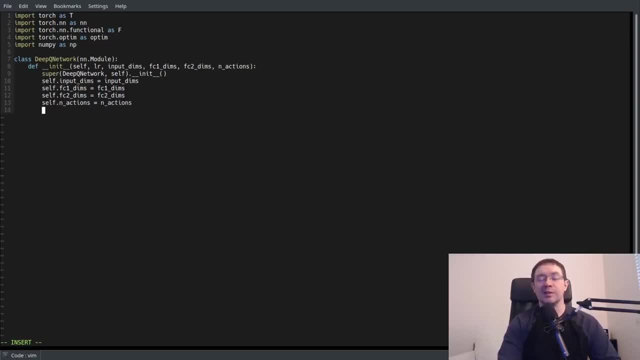 but you know, If we want to extend the functionality later, We're gonna have to add this stuff in later. so you may as well have it now and we arrive at our first layer of our deep neural network and that'll take star. selfinput dims has input and will output selffc1 dims. 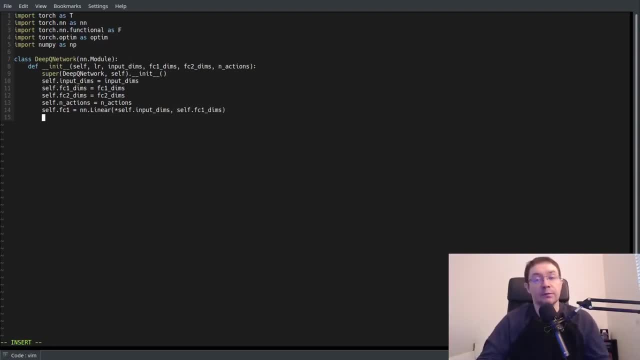 and the star selfinput dims idiom if you're unfamiliar with it is a way of unpacking a list in this case. so we're going to pass in a list of the eight- basically of course, mine to eight- elements of the observation vector. it's a way of making a little bit more extensible so that, if you 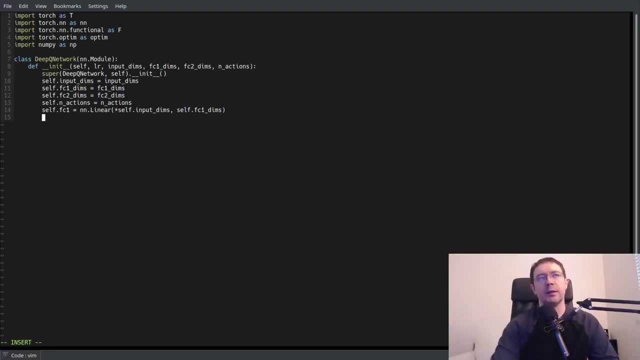 want to extend this to say a convolutional neural network that will facilitate that. or rather more specifically, if you want to extend it, to an environment that has a two-dimensional matrix as input, and so the second linear layer will take fc1 dims as input and output, fc2 dims. 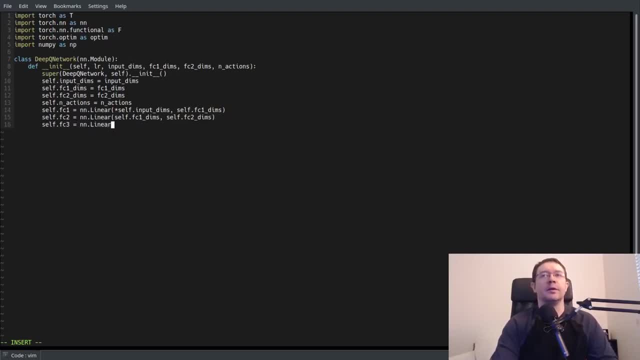 and fc3 is the output of our deep neural network, and i'll take fc2 dims as input and output. what number of actions? and we can go ahead and call it selfinactions. so the reason is that a deepq network is an estimate of the value of each action given some set of states. 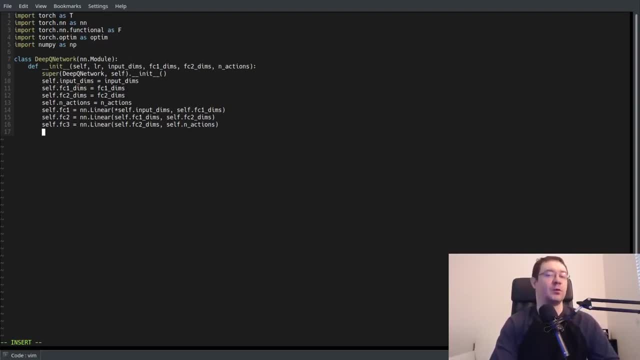 so if i do the agent performance, what action? what is the expected future reward, given it is in that state and follows its policy? we also have an optimizer. in this case, we use atom and we're going to pass in the learning rate and we have a loss function. 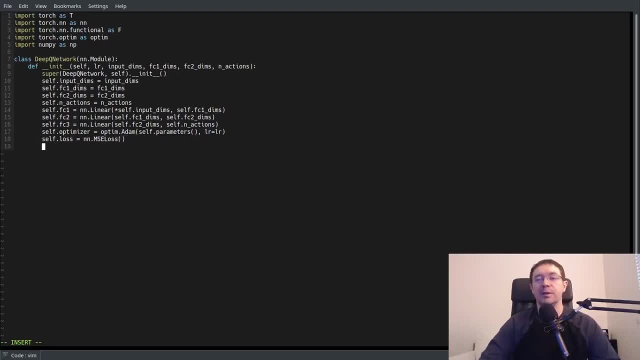 that's mean squared error loss, because q learning is basically kind of like a linear regression, where you're going to try to minimize the distance, or rather you're going to fit a line to the delta between the target value and the output of your deep neural network. oh, and something i didn't 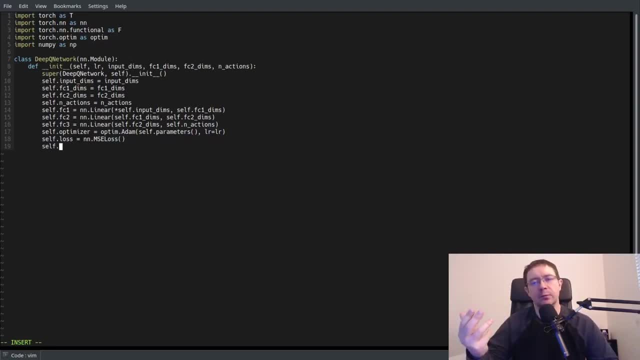 state before is that this is a simple representation of a deepq learning agent. this isn't the full that we cover in the course, where we have both a replay network and a target network, we're just going to use the replay network for this. we're not going to use the target network because it 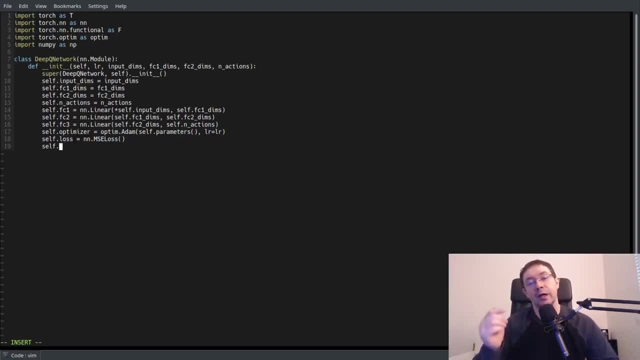 turns out. in this case, the target network isn't really required. however, a replay memory is almost certainly always required, which you learn in the course, and i have a free preview here on the channel where you can see the results of running a deepq network without a replay memory, just using 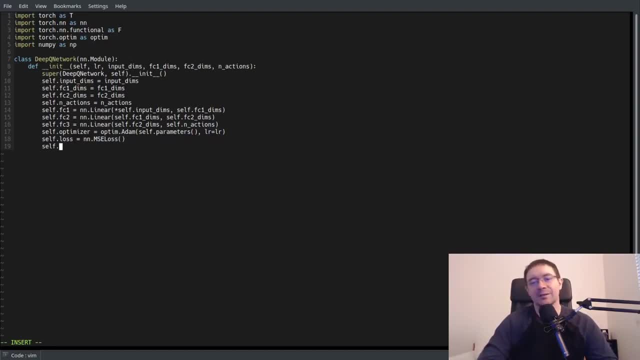 regular temporal difference learning and surprise, surprise, it's highly unstable. it kind of learns for a few moves and then forgets everything it learned. and i cover all of this in the course as well as a little bit in that video on the free preview. we also need a device, and this takes 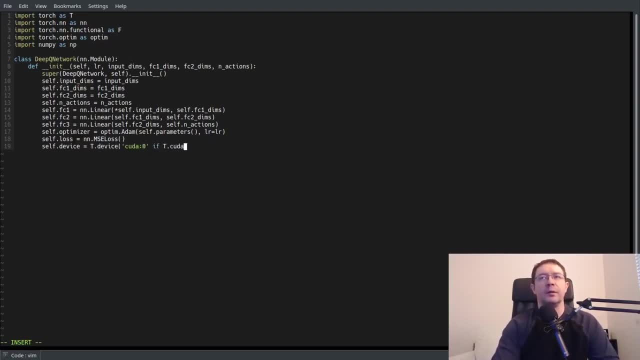 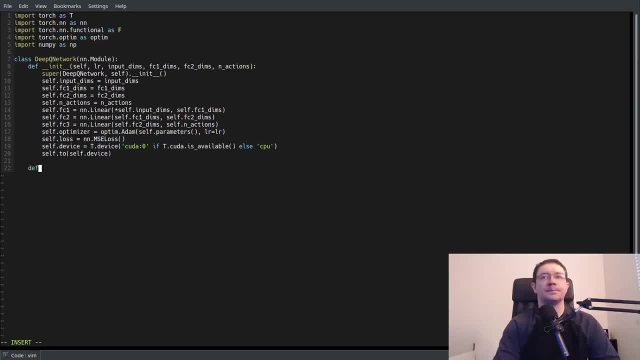 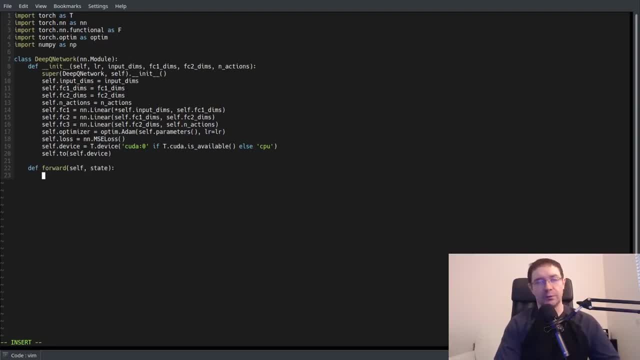 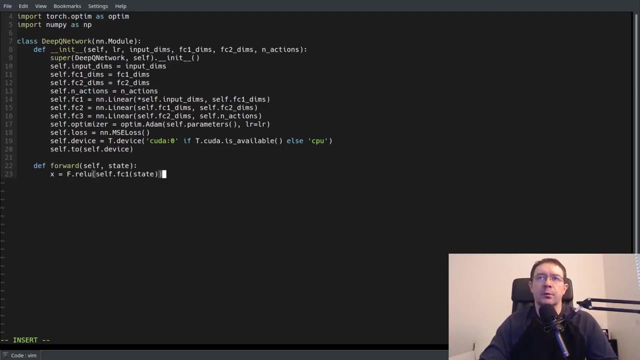 propagation, because you need, you know, to define your, say, activation functions. so we want to say cellfc1 state. so we want to pass the state into the first. you know, let's blow up the text a little bit for you guys. so we want to pass the state into the first fully. 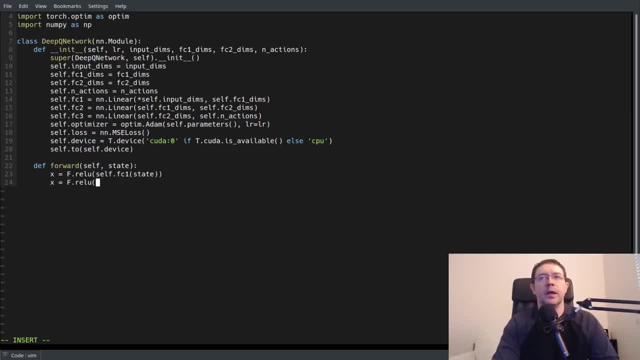 connected layer and then activate it with a value function. and then we want to pass that output from that layer into the second fully connected layer and yet again activate it with the value function. and finally, we want to pass that output to the third fully connected layer, but we don't want to activate it, and then we want to return that. 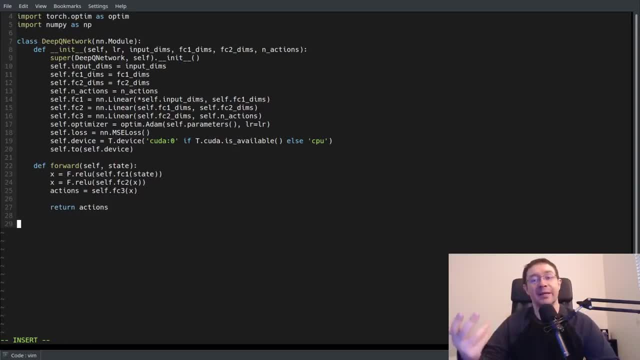 value and we don't want to activate it because we want to get the agent's raw estimate. we don't want to use, say, a row you function, because the estimate of the present- the present value of the feature rewards- could very well be negative, so we don't want to row you. it could very. 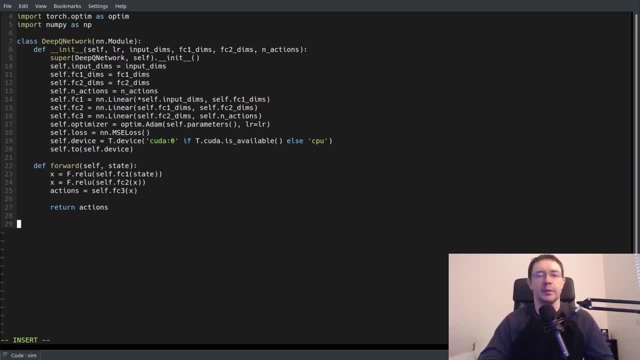 well be greater than one. so we don't like a sigmoid or a tan hyperbolic, something like that. so we don't want to activate it, we just want to get the raw number out, and that is it for a deep queue network class. the main functionality lives in the agent class and that doesn't. 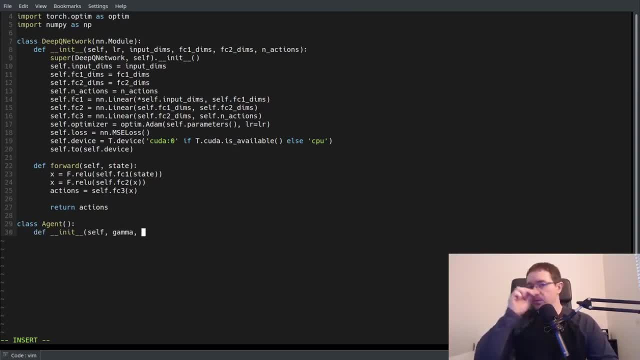 derive from anything. so we have the pass in hyper parameter gamma. that uh determines the weighting of future rewards. the epsilon, which is the solution to the epsilon, the uh- excuse me, the explorer exploit dilemma. you know how often does the agent spend exploring its environment versus taking the best known action? and that has to be some finite value because you never know if you. 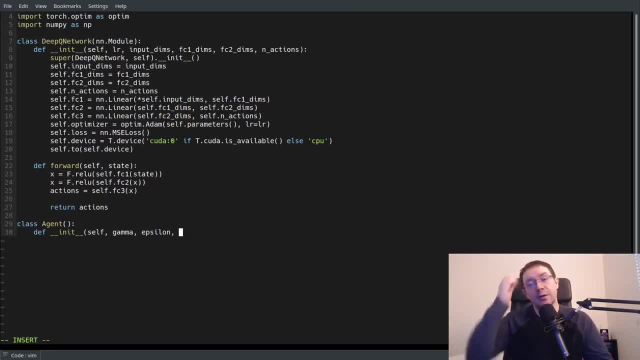 have a complete model of your environment. you know, how can you ever be sure that what you think is the best action actually works? and that's what we're going to do today. we're going to go ahead and actually is answer is you can't, so you got to keep exploring, and that is determined by a parameter. 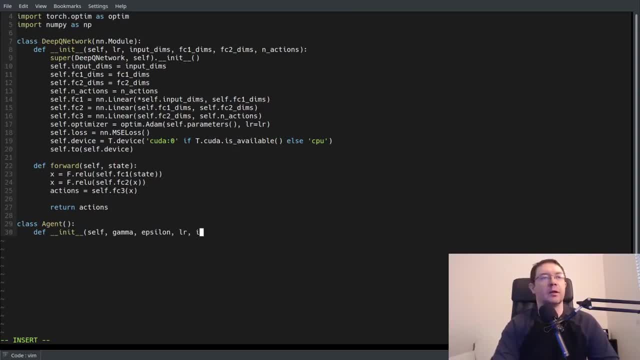 called epsilon learning rate to pass into our deep neural network. input dims: a batch size, because we're going to be learning from a batch of memories: number of actions and max memory size. as i said earlier, we're going to be using a memory. we use something like a hundred thousand um an epsilon. 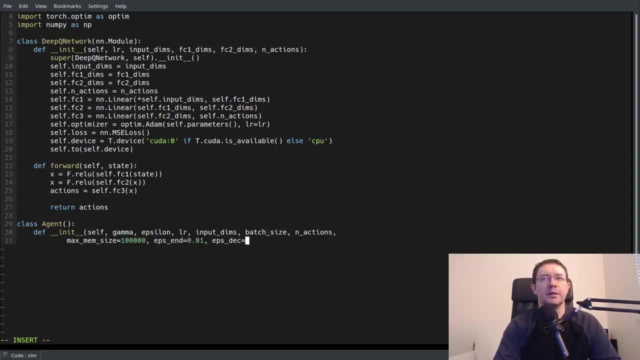 end will default to zero point, zero one and an epsilon decrement of five by ten to the minus four. so this is the parameter that tells us by what to decrement epsilon with each time step. you can do a multiplicative dependence, you can do one over a square root, you can do any. 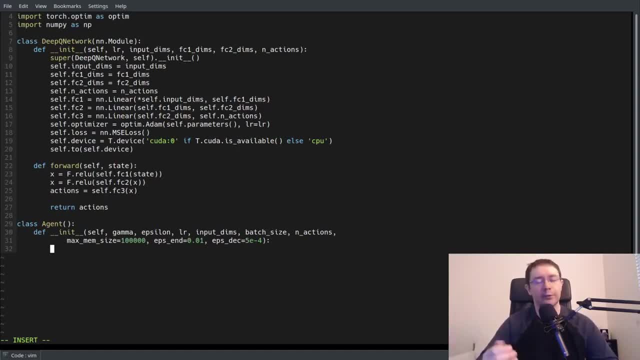 type of uh decrement you want. i'm just going to use linear, linear. we're going to subtract off a constant factor with each time step all the way down to the minimum. it doesn't really matter. it's one of the least important hyper parameters. the main thing is that you give it some time of. 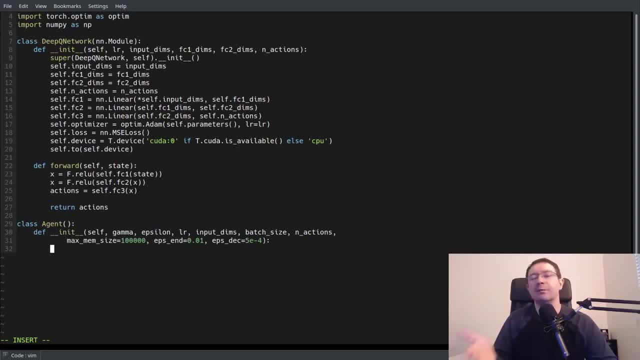 acting randomly and then decay it over time to a minimum value and leave it at a minimum which is non-zero, some finite value. so of course we want to save all of these variables and we also have what's called an action space: i in range, in in range- that won't work- and actions. 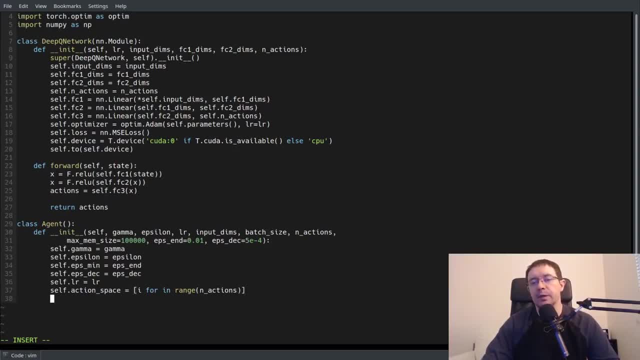 and this is just going to be a little bit more complicated, but it's going to be a little bit more complicated, but it's going to be a little bit more complicated, but it's going to be a little bit more. this is just a list, comprehension that tells us the integer representation of the available. 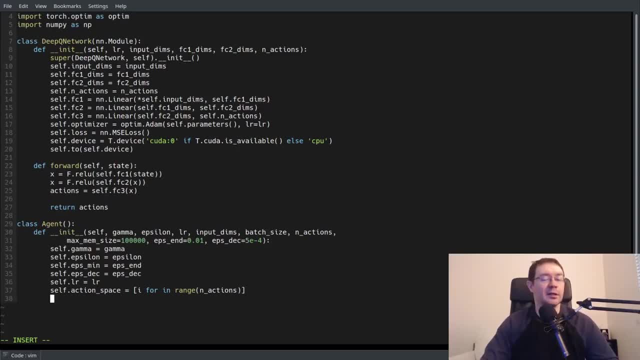 actions and the reason is because we're going to use this later in the epsilon greedy action selection just makes it easy to select an action at random, as you will see in a moment. so we'll say max mem size as our memory size say our batch size. 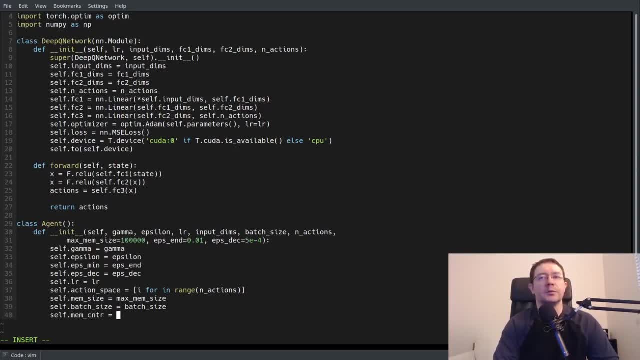 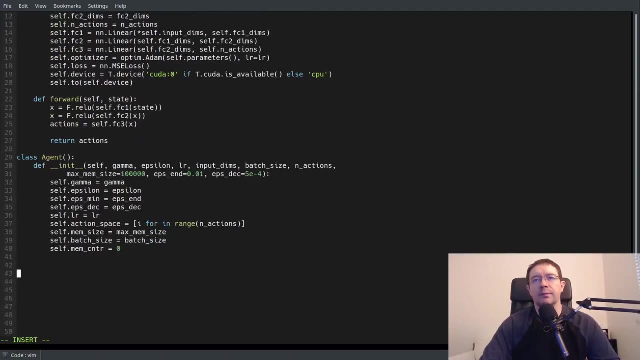 we need a memory counter, and the point of that is to keep track of the position of the first available memory for storing the agent's memory. and we also need the. can i scroll down a bit? let's do that. we also need the evaluation network, so we'll say selfq. 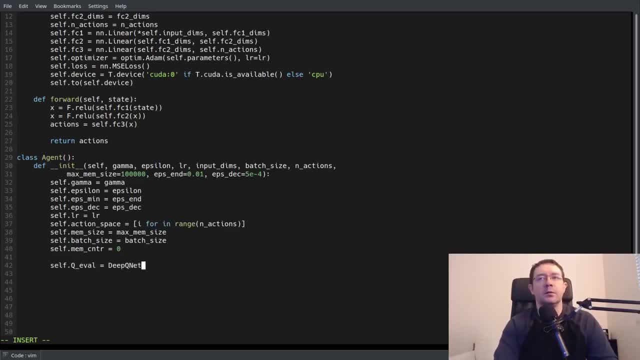 eval equals deep q network and we'll pass in the learning rate number of actions. we need to do that. we need the input dims. we need fc1 dims. we're going to default this to 256. c2 dims: 256. let's tab that over a bit and you can play around with this. it's not super critical. um, i mean it to some. 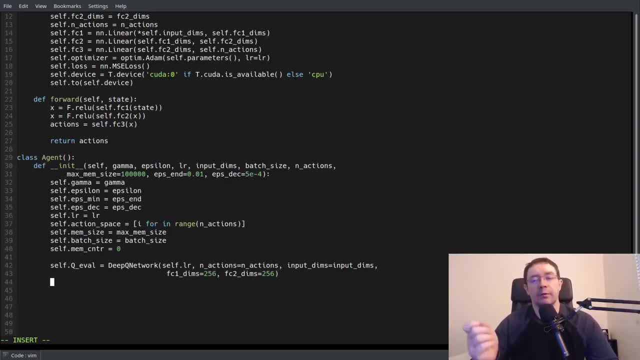 extent is, but it will function for a wide range of neurons in the fully connected layers. in addition to the deep neural network. you also need some sort of mechanism for storing memory. now many people will use something called a deck or a dq, which is a, basically a list, in python. 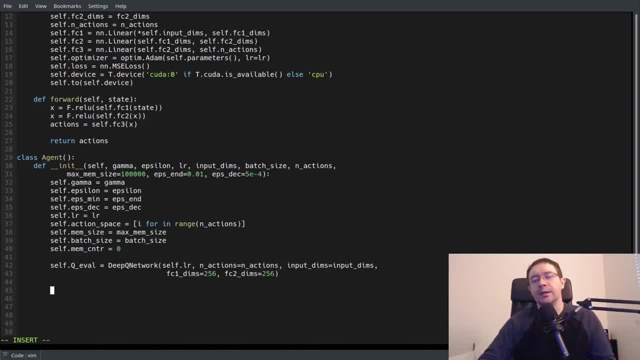 a linked list, so it's a dynamic memory structure and you pop things off one end and insert them in the other. um, i don't like doing that, because then you're going to store basically a collection of arrays anyway, and then you have to dereference it. so you have to say: you have to know which. 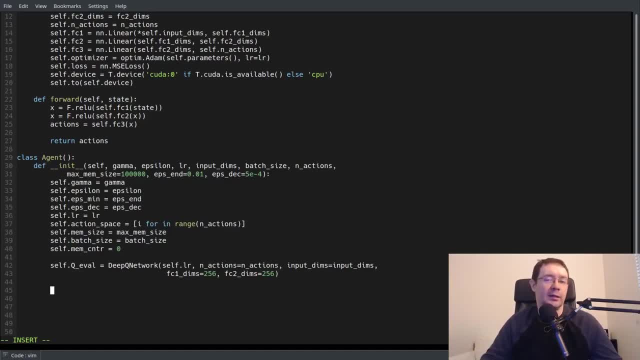 array you're in. i don't like doing that because you have to know the position of the of the dq corresponds to which array. so i just like saving them as named arrays anyway, because it's much cleaner and more more easy to read. so what i mean specifically is: state memory equals mp zeros. 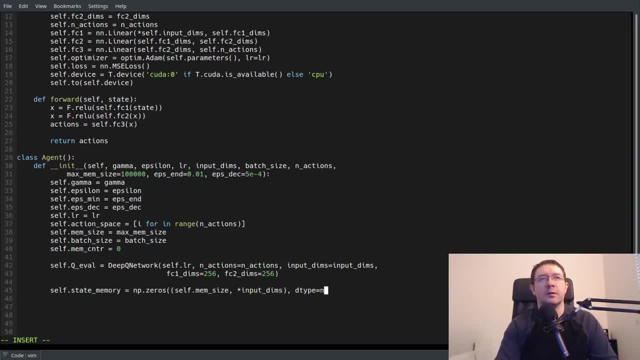 selfmem size by star input dims and we're going to use np float 32 as our data type. uh, the data is rather particular about data types. it enforces some degree of type checking, which is a good thing. it can be a little bit annoying at first, but once you're aware of it it really saves your. 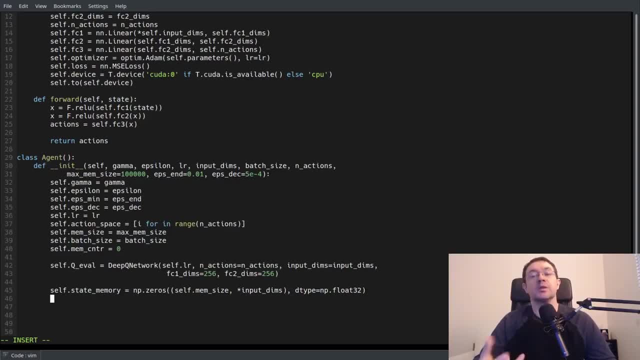 bacon later on because you lose some stuff when you go from one level precision to another. so make sure that things are nice and consistent. it's quite handy and we also have a memory to keep track of the new states the agent encounters. so what the agent wants to know for the temporal difference update rule is: what is the value of? 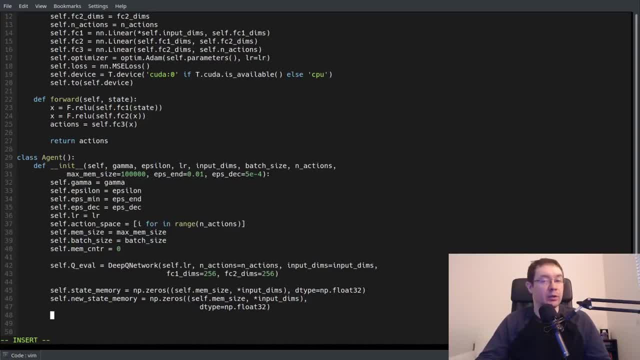 the current state, the value of the next state, the reward it received in the action it took, and to get that you have to pass in a memory of the states that were generated and the state that was received in the action it took and you can keep track of what you did and the states that were generated and the state that wasド. 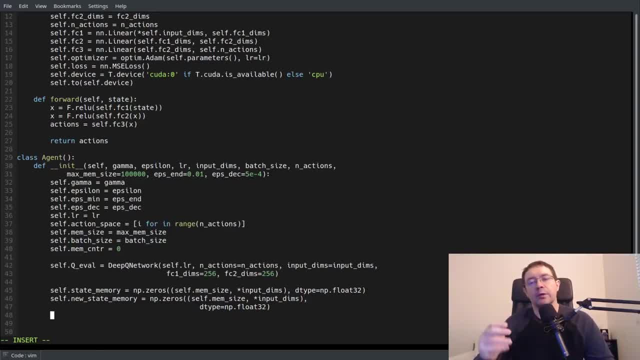 resulted from its actions, because, remember, deep q learning, if you're not aware, is a model, free, bootstrapped off policy learning method. what that means is we don't need to know anything about the dynamics of the environment, how the game works. we don't need to know anything about that, we're. 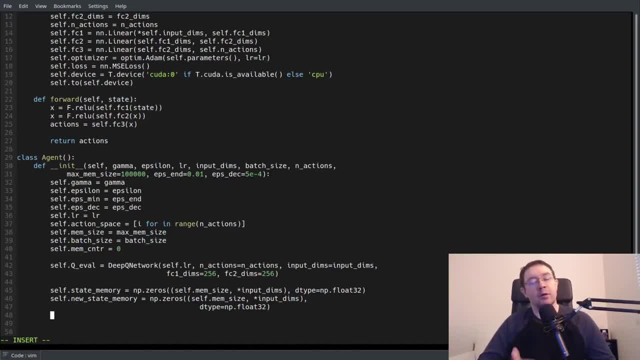 going to figure it out by playing the game. uh, that means model free. bootstrapped means that you are going to construct estimates of action value functions, meaning the value of each action given you're in some state based on earlier estimates, you're using one estimate to update. 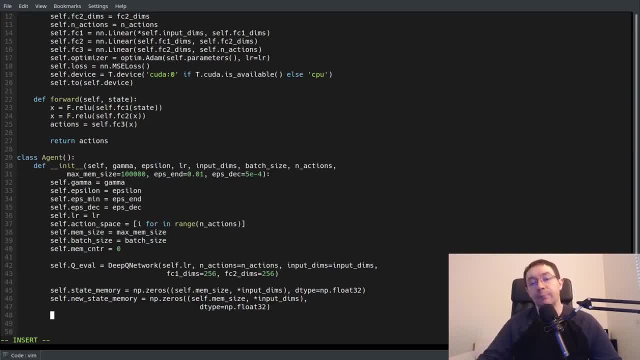 another. in other words, you're pulling yourself up by the bootstraps off policy means that you have a policy that you use to generate actions, which is epsilon- greedy, meaning that uses hyper parameter that we defined up here, epsilon, to determine the proportion of the time that you spend taking. 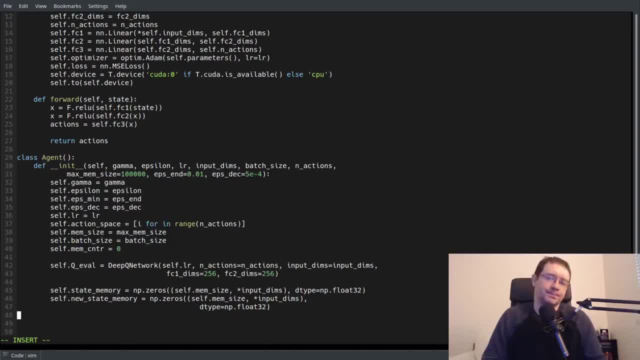 random versus greedy actions and you're going to use that policy to generate data for updating the purely greedy policy, meaning the uh agents estimate of the maximum value function, action value function. sorry, so it is off policy in that sense. so a lot of buzzwords there, more that is covered in the course, but that is the. 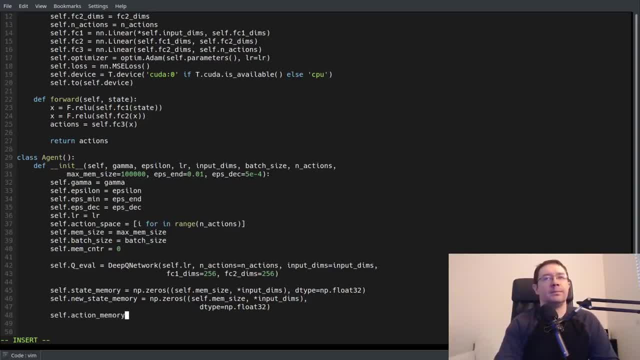 gist of it. so we also need an action memory and that is an array of numpy zeros, selfmem size, and we use np in 32. uh, just a set of integers, because our this is a discrete environment. deep learning doesn't really work for discrete environments, so you can do, sorry, discrete. 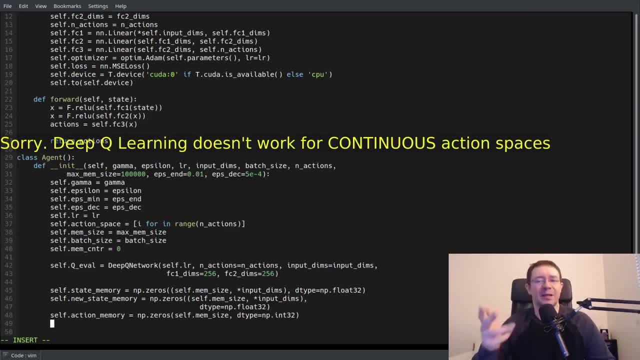 action spaces. so you can do some tricks to kind of get around that, but you know they don't work as well. we need a reward memory and that is shape, mem size and uh d type of np float 32, and so these will be floating point numbers because they can be fractional numbers, they can be 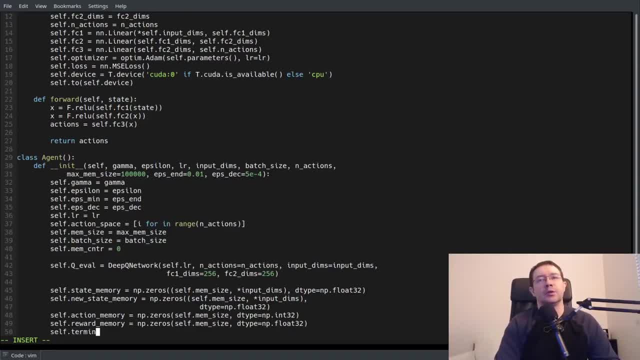 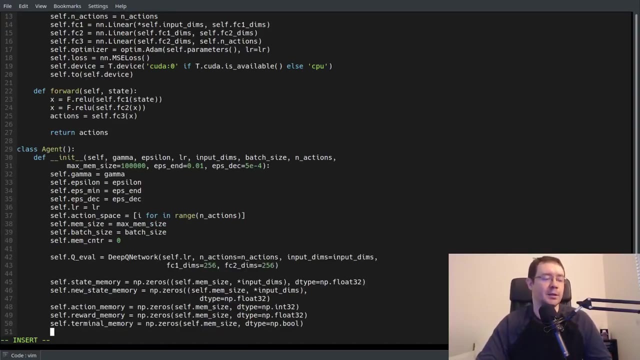 decimal point numbers you. we also need a terminal memory, and the point of this is sorry. the point of this is that the value of a terminal state is always zero, so the reason behind that is simply put: if you encounter the terminal state, the game is done right, and so there are no. 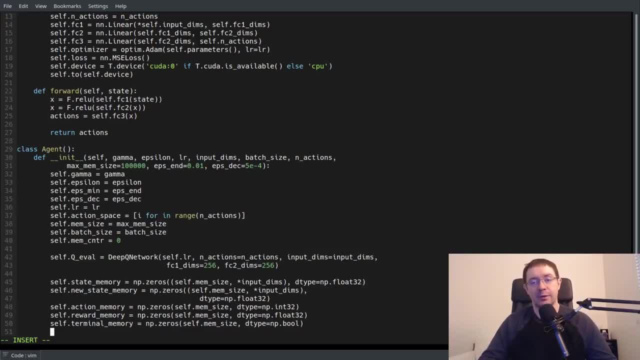 feature actions until you reset the episode. but when you reset the episode you're in the initial state, not the terminal state. so the future value of the terminal state is zero. so we need a terminal state is identically zero and so we need some way of capturing that. when we tell the agent to: 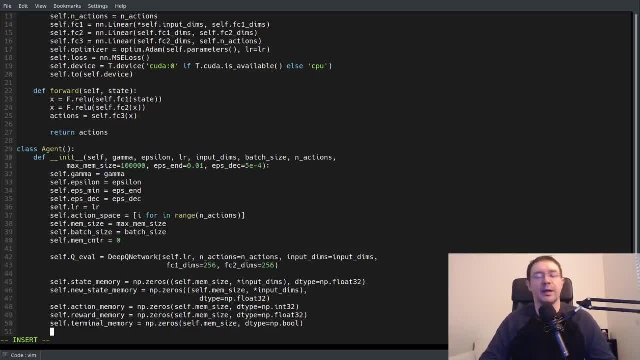 update its estimate of the q value, the action value function q, and that is facilitated through the terminal memory and we're going to be passing in the done flags from our environment, and it is therefore type np dot bool, and that allows us to use it as a mask for setting the values of the. 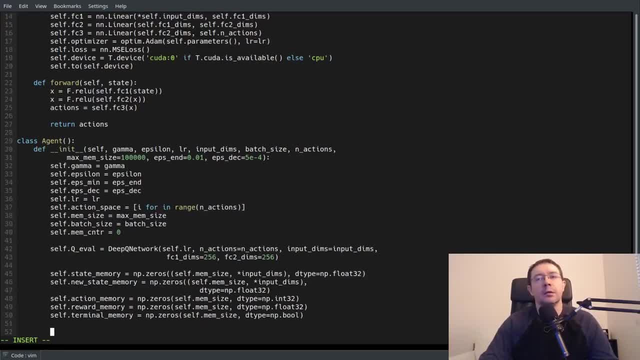 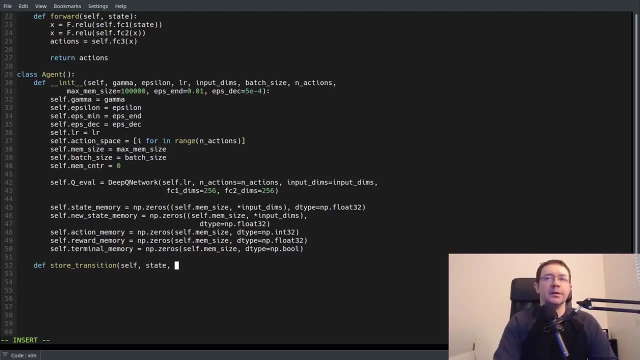 next states to zero later on, which we'll see in the learning function. that is it for our constructor. next we need an interface function to store one of those transitions in the agent's memory so that'll take a state action, reward new state and done. flag as input. 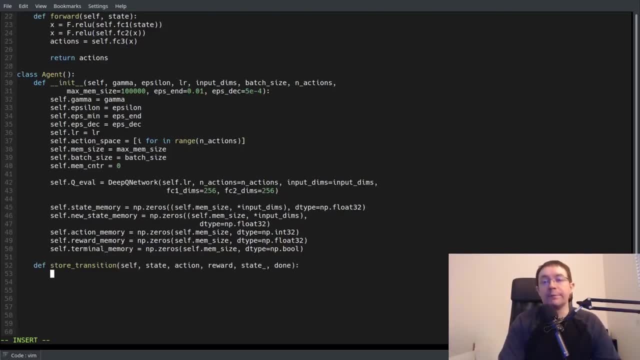 now i occasionally call this terminal or sometimes done. but the first thing we want to know is: what is the position of the first unoccupied memory? so, index, selfmemory, counter, modulus, mem size, now, uh, using the modulus here has the property that this will wrap around. so once we go from memory zero up to 99, 999, that hundred thousand memory we go to store, we'll go. 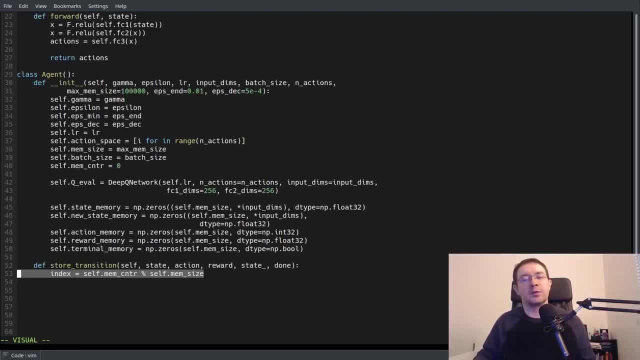 all the way back in position zero. so we rewrite the agent's earliest memories with new memories, and that's because the memory is finite. if you're using a memory that's finite, you're going to have to use a memory that's finite. if you're using a deck or a dq, then you're just going to be popping stuff. 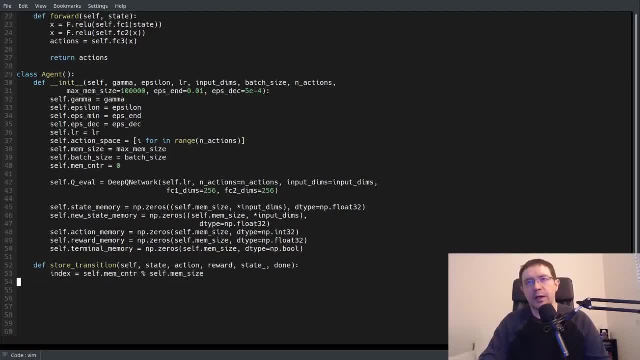 off the end once you get beyond the limitation- the size of the agent's memory. so now that we know where to store it, let's go ahead and store it. action memory dot. now, this is part of the reason I am redoing it. but first you've got to increment the memory. 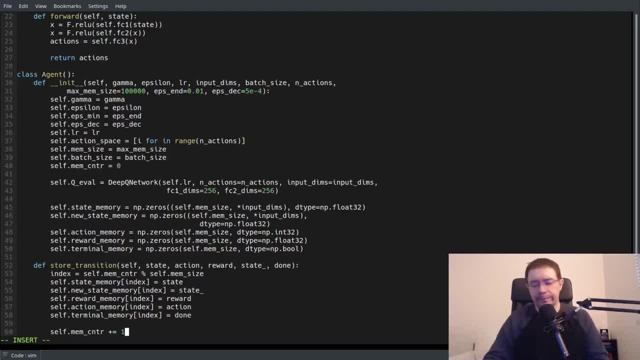 counter by one to let yourself know that you have filled up a memory, and this is part of the reason I am redoing this. so this action memory here. originally I had gone from a one-hot encoding where you take an integer and represent it as an array of zeros, with a one corresponding to the. 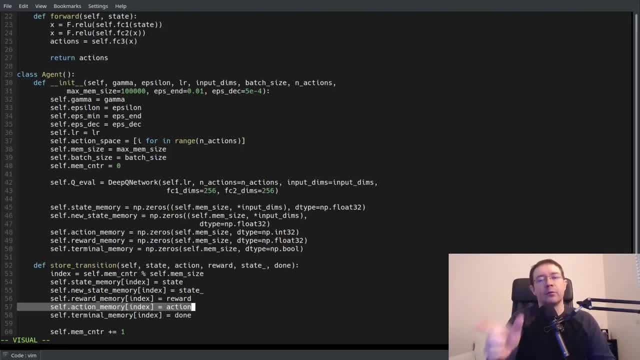 position of the integer. so you have four actions. you have an array of four elements: zero, one, two and three, and if the agent took action four, the one-hot encoding representation of that is zero, zero, zero one. 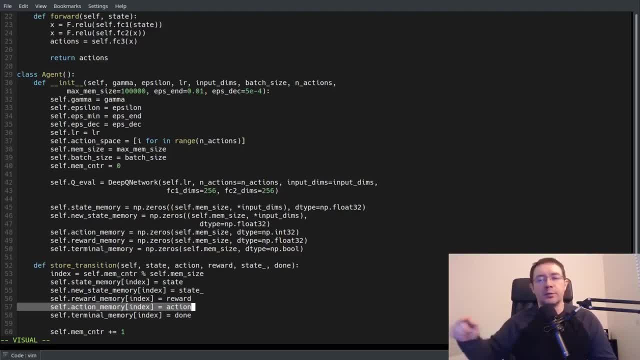 in an array, if it's action one, it'll be zero, one, zero, zero, so on and so forth. and then I went from that one-hot encoding back to the integer encoding in the learn function, and you know this was done way back in October of 2018, and I 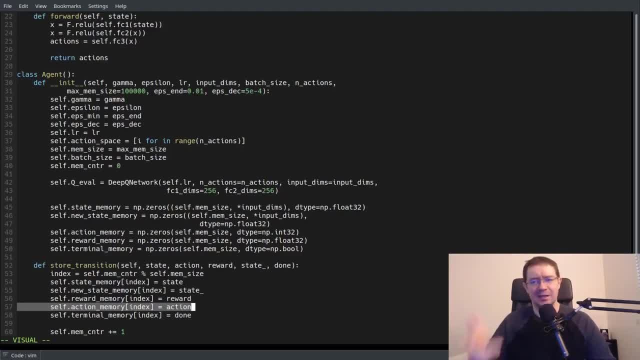 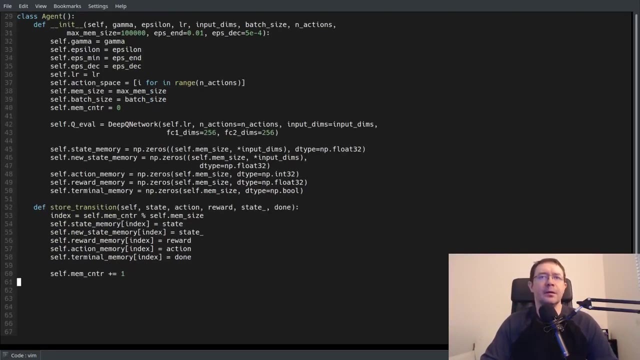 can't really remember the reason for doing that. suffice it to say it's dumb and it led to some issues with people's understanding, you know. and so I no longer want to use that way of doing things and in fact I moved on beyond that, so we're not going to do that anymore. just keep that in mind. 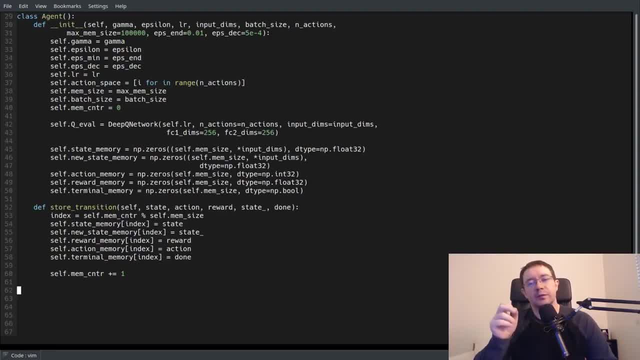 so the next thing we need to do is a function for choosing actions. so the agent has to have some function to choose an action and that is based on the current state of the environment. sorry, we'll call the call it observation, and you'll see why in a second. so the observation of the current state. 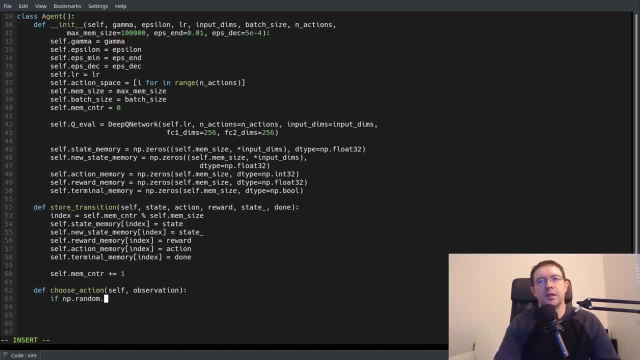 of our environment, and the first thing I'm going to do is take a random number and say: if it's less than epsilon, sorry, greater than epsilon, epsilon. then if it's greater than epsilon, we want to take the best known action. so what we? 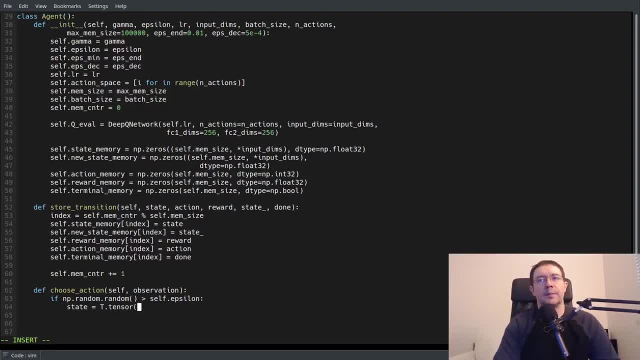 have to do is take our observation, turn it into a pi torch tensor and send it to our device, because everything, the entire network, lives on our device. so we have to send the variables we want to perform computations on to our device and we need this bracket around. 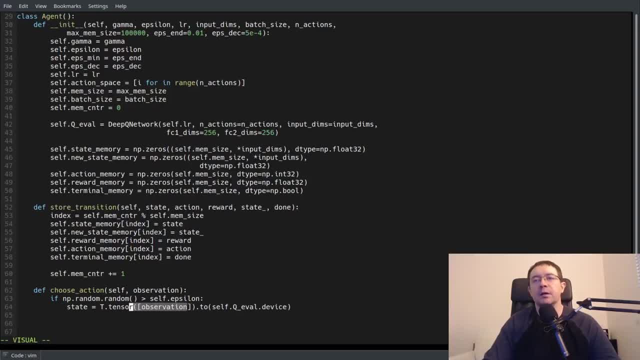 the observation because of the way the deep neural network is set up. and so then we pass that state through our, our, our, our, through the forward function, and then we want to get the argmax to tell us the integer that corresponds. 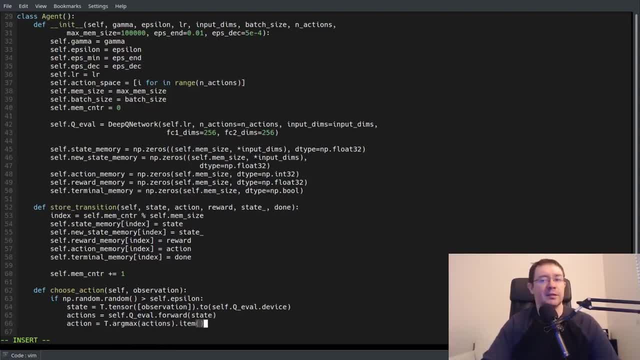 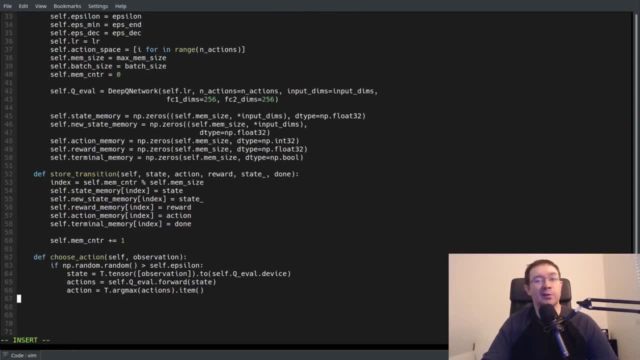 to the maximal action for that set or state and you have to dereference it with not item, because it returns a tensor and we're going to be passing this back to our environment, which only takes integers or numpy arrays as input. Now, if it, 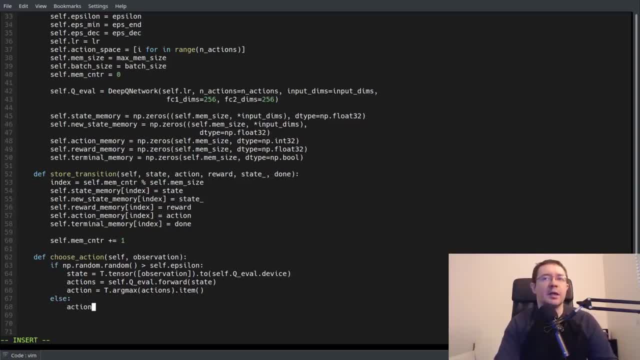 is not greater than epsilon, meaning if it's less than or equal to, then we want to take a random action and we'll just do a random choice from the agent's action space and regardless of how you select the action, you want to return it. 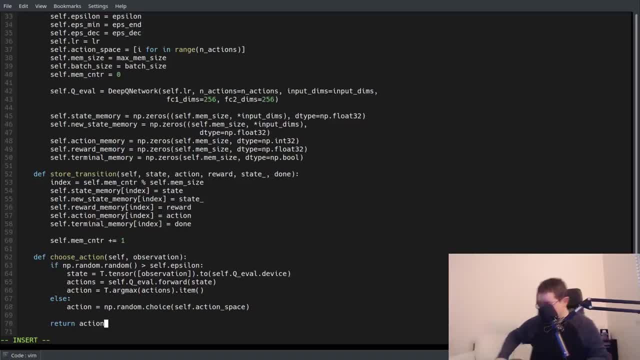 One moment. the kitty cat is scratching at the door. let me let her in, Say hello, kitty Meow, She looks very pleased. Okay. So now that we have a mechanism for choosing actions, we can think about how the agent is going to learn. 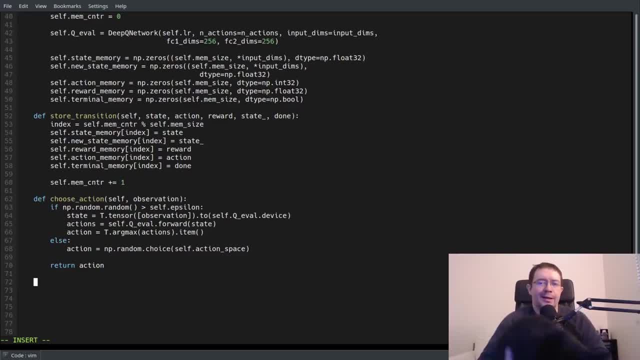 from its experiences. So sorry, cat, you gotta go, She's in the way. So we do that through a function called learn and that does not take any inputs, And right away we're faced with a bit of a dilemma, and the dilemma 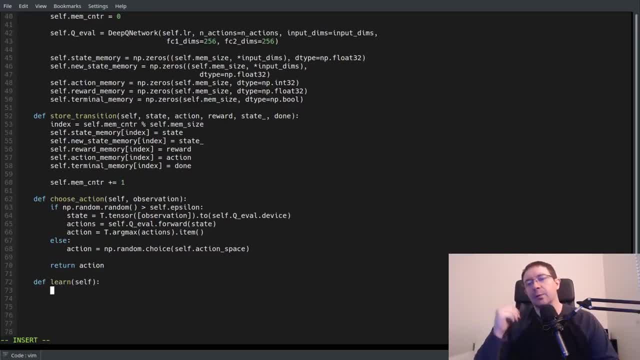 is if we, you know, we have this memory and it's filled up with a bunch of zeros which we can't really learn anything from, zeros. it's kind of stupid to try. So how do we deal with that? Well, there's a couple ways. 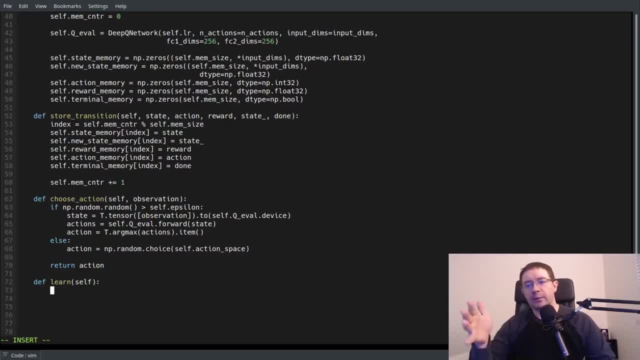 One way is you can let the agent play a bunch of games randomly, you know, until it fills up the whole entirety of its memory, And then you can go ahead and start learning. That's one possibility. You know, we're not actually selecting actions intelligently. 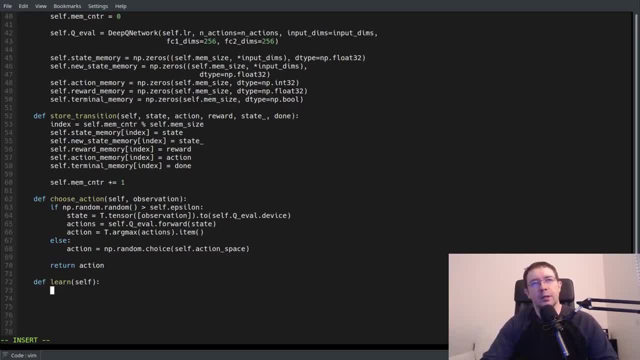 we're just doing it at random. That's one possibility, And another one is to simply not do that, but to start learning as soon as you've filled up the batch size of memory, And so we can facilitate that. that's what I'm going to choose to do. 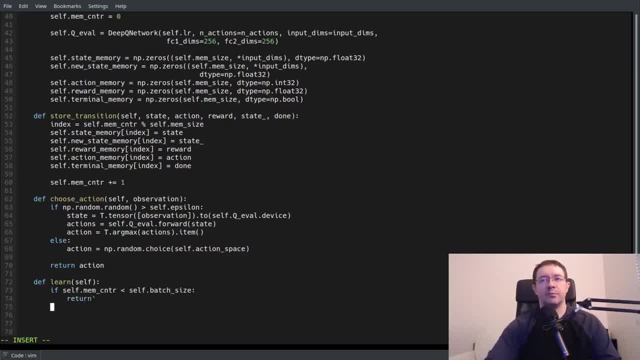 By saying: if our memory counter is less than the batch size, just return. So we're going to call the learn function every iteration of our game loop and, you know, if we have not filled up our at least the batch size of our memory, just go ahead and return. 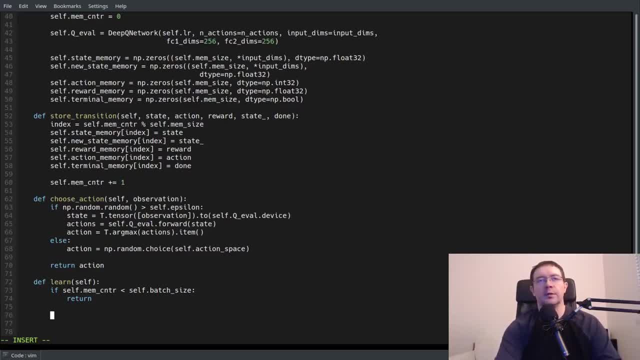 don't bother learning, no point in it. So the first thing we want to do, in the event that we are going to try to learn, is zero the gradient on our optimizer, And this is particular to PyTorch. you don't have to do this in, say, Keras. 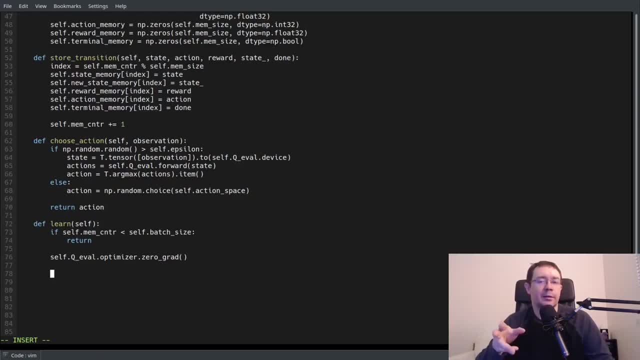 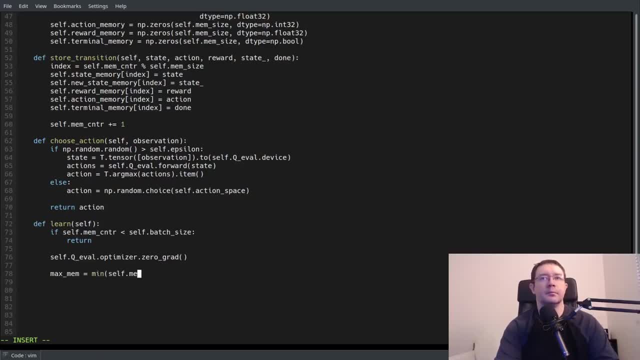 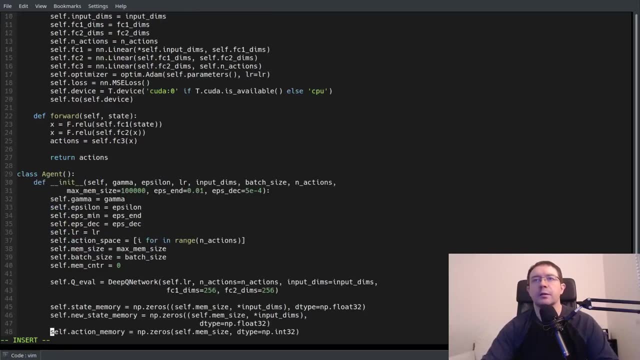 So we want to take the minimum of either the memcounter or the memsize. Memsize, is that what I called it? Let me double check: Selfmemsize: yep, So it's the minimum of either the memcounter or the memsize. 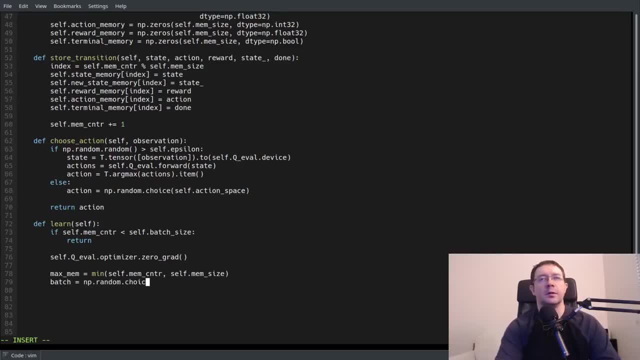 I'm going to say: batch equals mp. random choice Max mem selfbatch size. replace equals false. Now we want the replace equals false. because we want the replace equals false. we don't want to keep selecting the same memories more than once. now, this isn't a problem if you. 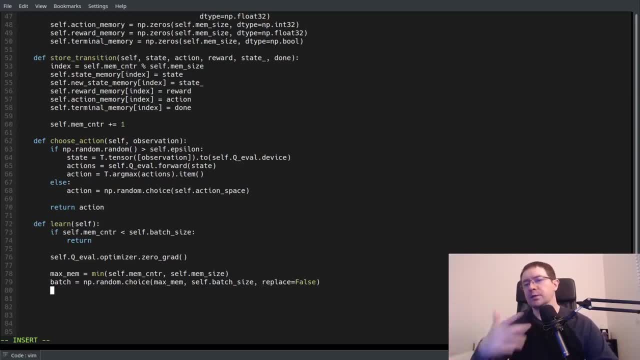 have stored 50,000 memories or a hundred thousand memories, but it is a problem if you stored, you know, 32 memories or 64, whatever you know batch size or some small multiple thereof. so you want to make sure that once you select a memory, you take it out of the pool of available memories. 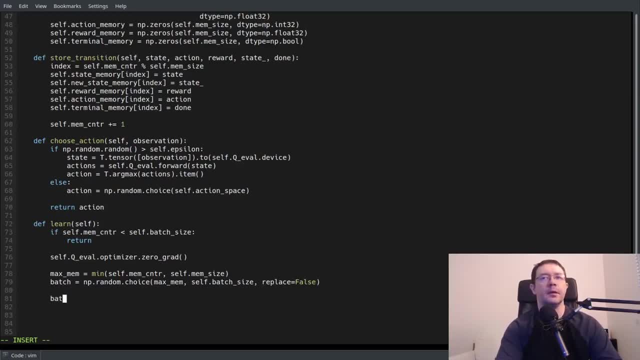 to select again. and then we need just something for bookkeeping, basically a batch index, and this was also a point of confusion on the github for my previous video. you most certainly need this batch index and you most certainly need the action indices to perform the proper array slicing, if you. 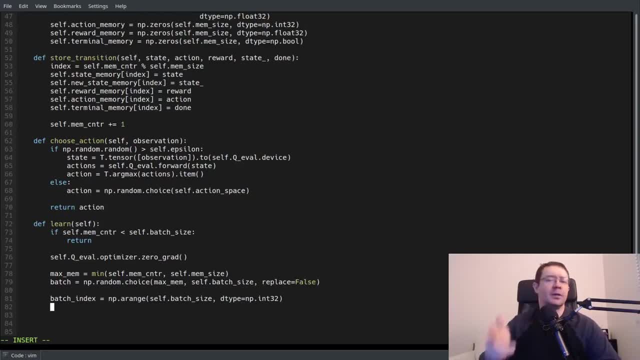 don't use them, you don't get the right thing, and I made a video detailing that in an earlier on, maybe a month ago, something like that. but yeah, you need this 100% certain on that, so I'm gonna, when I upload this code to github, don't forget to check that out, and I'll see you in the next video. 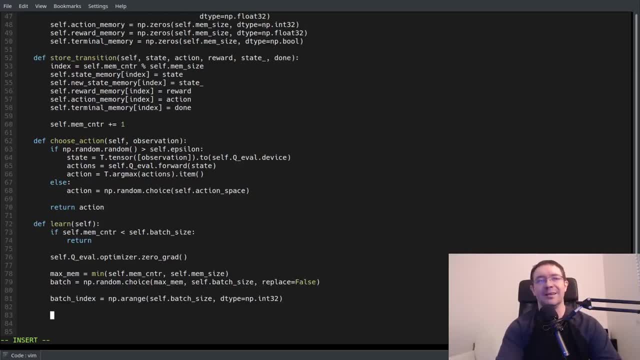 don't give me, you know, issues on this, because this is the way you do it. so state batch equals T dot tensor, self dot state memory dot to Q eval dot device. so what we're doing here is we're converting the numpy array subset of our agents memory into a PI torch tensor, and we also have to. 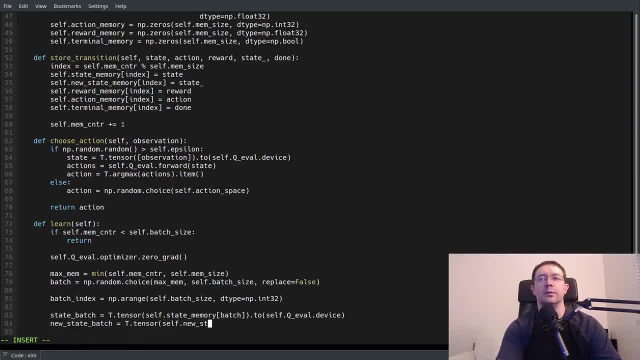 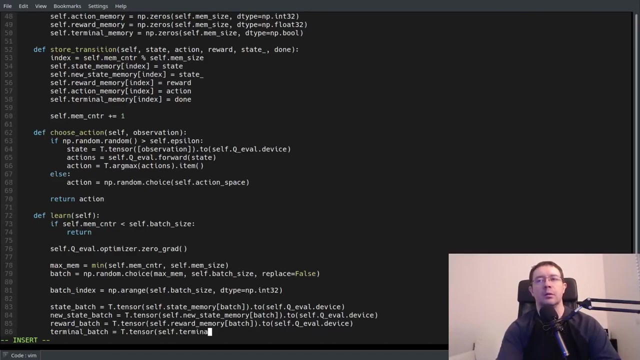 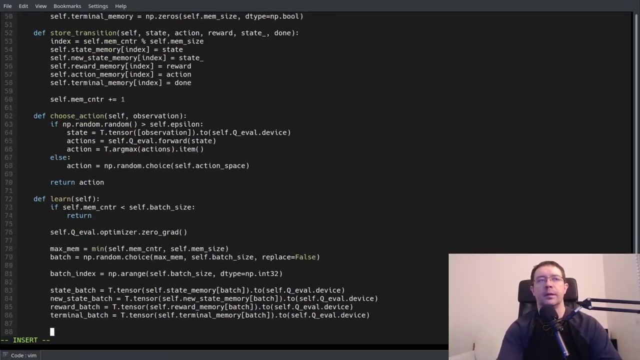 do the same thing for the new states, new state memory, sub batch to self Q eval device. we need the same thing for the reward batch. we'll say reward batch, eval dot device. and we also need the same thing for a terminal batch. and we do need an action batch. but that doesn't need to be a tensor, it can be a numpy array. so 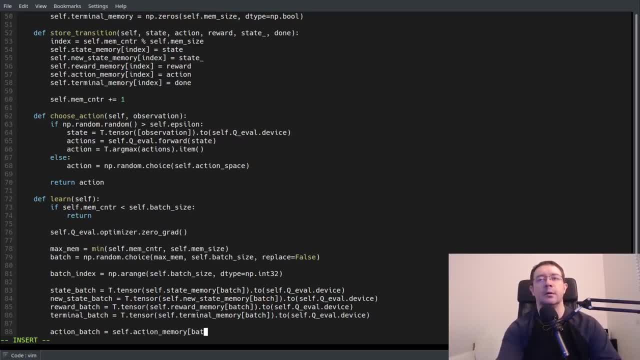 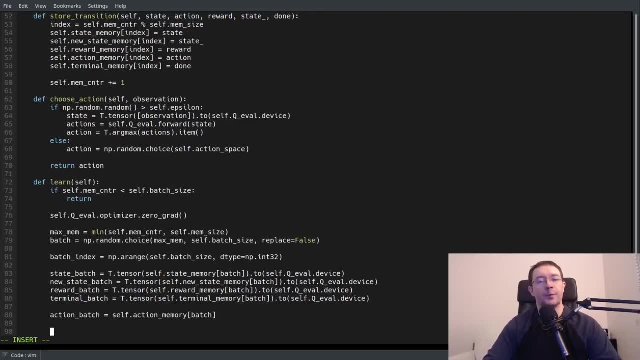 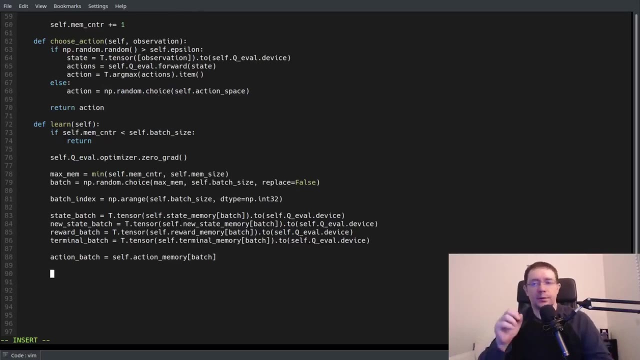 that is your self dot action memory sub batch. all right, so now we have to perform the feed forwards through our deep neural network to get the relevant parameters for our loss function. what do we do to that? we want to be moving the agent's estimate for the value of the current 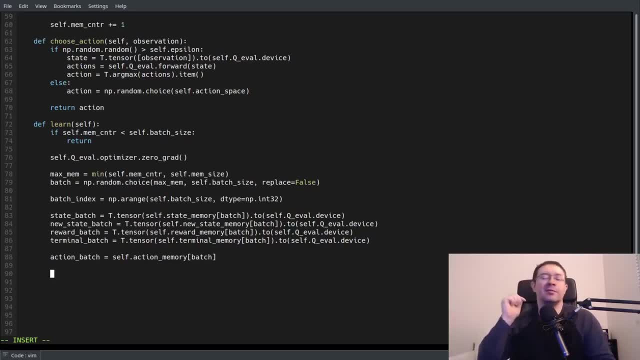 state towards the maximum value for the next state. so in other words, you want to tilt it towards selecting maximal actions. and we do that by saying q eval equals 어 dot, Q eval dot forward boundt. we have to do the D referencing, we have to do the array slicing, batch index, Ac action and the reason. is, we want to get the default values of the actual batch element, then in the result, it would assume that the value is getting de-referenced out. if we set the over Yeon's smart too much, we'll just do the być heroic method. for now, please keep patience and thanks so much for watchingitaand I'll see you in the next video. bye-bye the next video, bye. 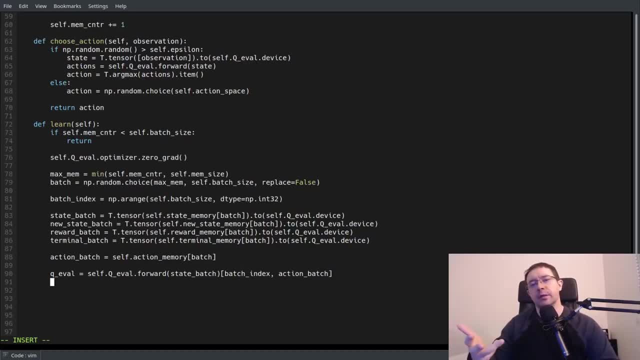 actions we actually took. those are the only ones we're really interested in. uh, you can't really update the values of actions you didn't take because you didn't sample those anyway. so we want the values for the actions we actually took at each set of our memory batch. 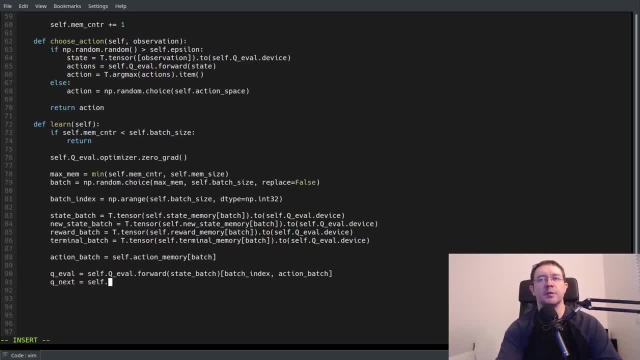 and we want the agent's estimate of the next states as well. forward new state batch and we don't need to do any dereferencing there. uh, we're going to handle that momentarily. we're going to get the max actions. uh, and if you were doing a target network, this is where you. 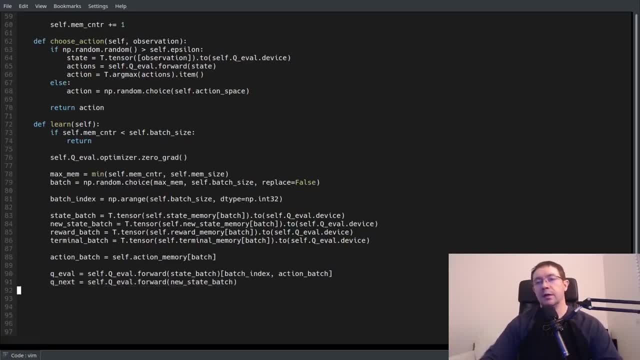 would use it. you would use it here. as i said, that is for more advanced stuff. we're not going to bother with that right now. the next thing we want to do is say the um, the values of the terminal states are identically zero, and then we want to calculate our target values. this is where we're. 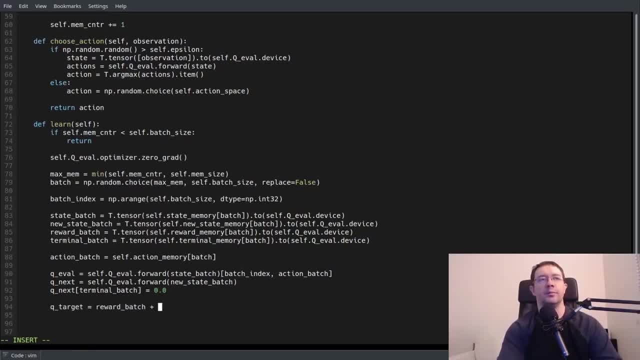 going to update our estimates towards you and that's the reward batch plus self dot gamma, that's our discount factor times the max over um q, next along the- uh- it's dim, sorry, not axis- along the action dimension and the zeroth element, because the max function returns. 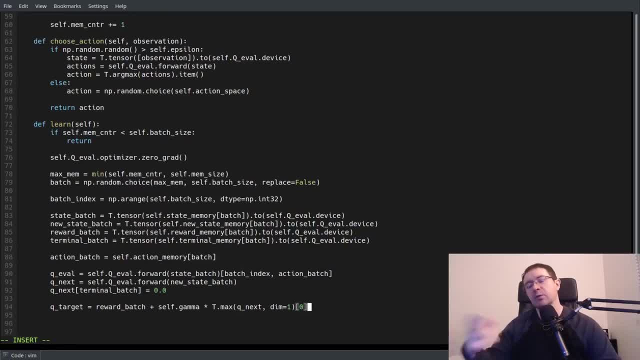 the value as well as the index. so it's it returns a two-pole. we want the zeroth element, which is the value, so this is the maximum value of the next state, and we're going to do that here, and that is the purely greedy action and that is what we want for updating our loss function. 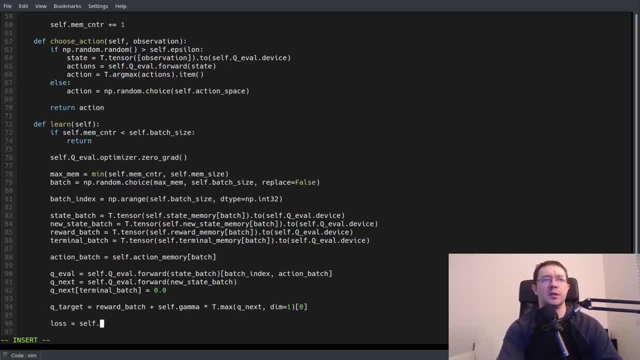 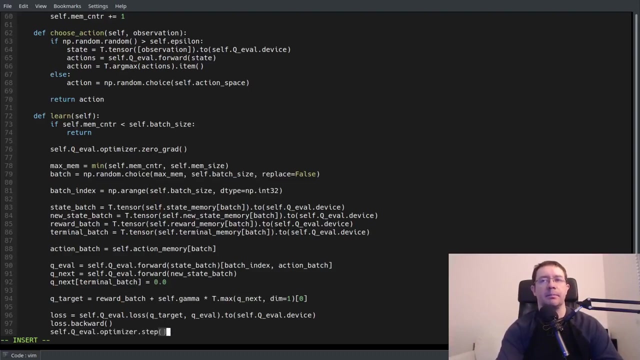 so our loss then is just the q eval dot loss, q target, q eval dot to self dot, q q eval dot device, and you want to back, propagate it and step your optimizer, eval optimizer, to the better estimate of the result, to be just this very top one here. so that's really it, we'll be. 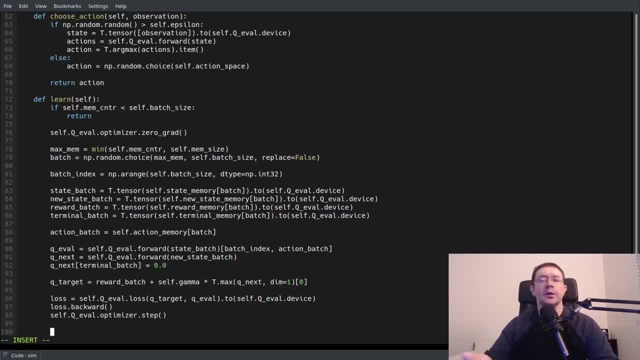 doing. what that is we're going to do here is we're going to take our map structure here and call it just the new max point規을 faculty class, which in this case is for student data, and so we're going to double check that out and then we're more than happy to add that to theОb reptile step. and that is it for the nuts and bolts of the learning. the next thing we have to handle is the epsilon decrement. so each time we learn we're going to decrease epsilon by one, so we'll say selfepsalon by one unit of epsilon decrement. 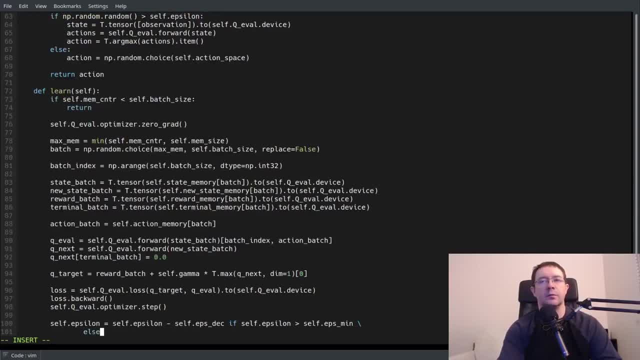 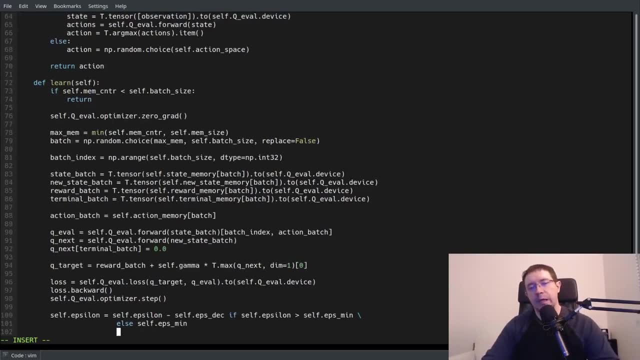 min, otherwise set it equal to EPS min and that is your learning function. and this is the simplest possible implementation of deep Q learning you can really do, and it is only you know about a hundred lines of code. you know less than that if you count just significant lines of code. but this: 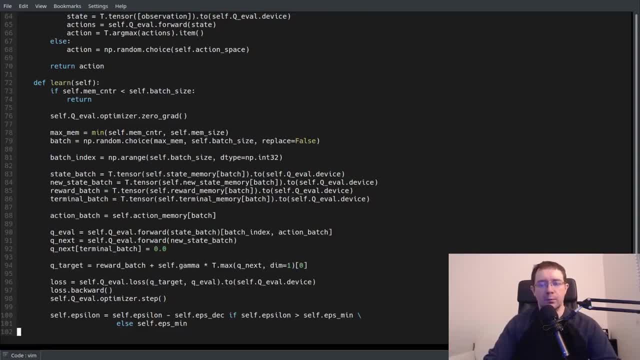 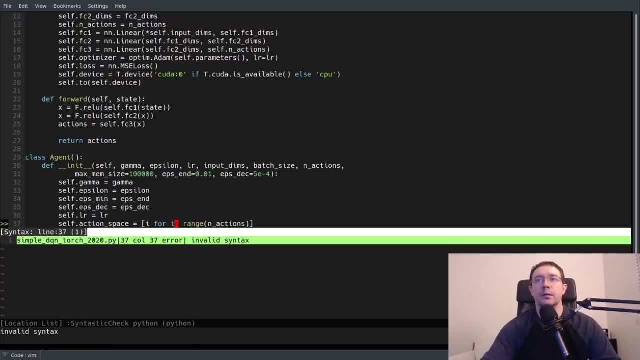 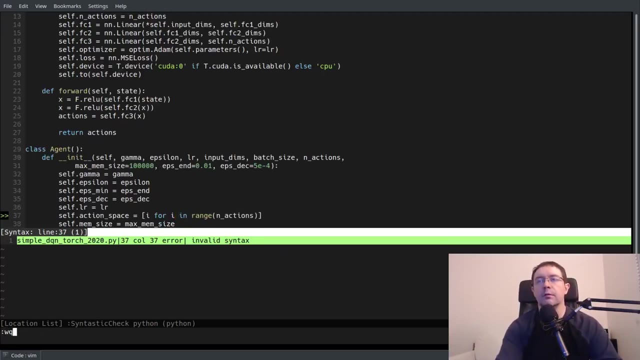 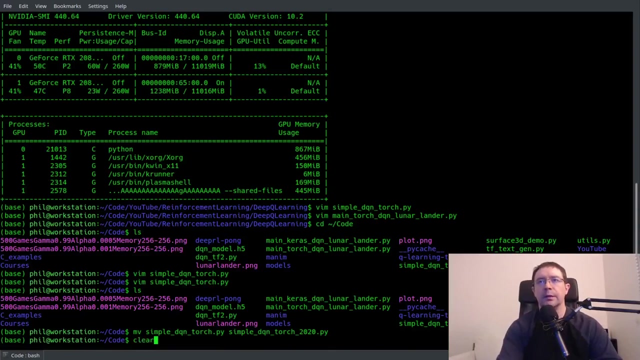 is pretty much it, folks. so we are done with the agent, and now we have to worry about fixing our syntax errors. it's on this line here for uh, insert I in range. there we go, and so let's go ahead and clear all of that. so now we're ready to handle the main file, so let's just vim main. 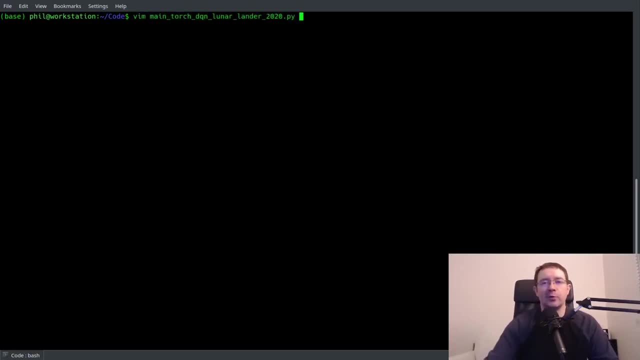 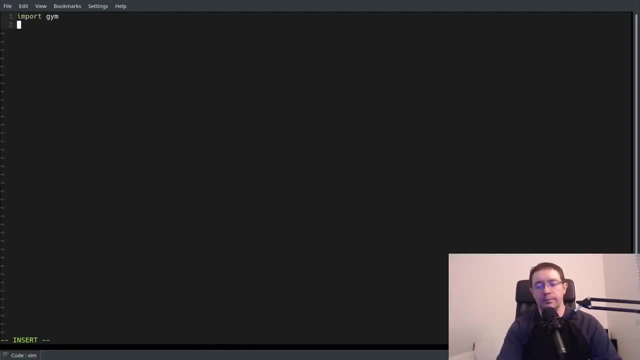 torch dqn lunar lander 2020, because this is the new version and we start with our imports. we'll need Jim. now- let's, I can increase one more- so we'll need Jim. we will also need our agent from simple dqn torch 2020 import agent, excuse me, uh- from utils import plot learning, and this is 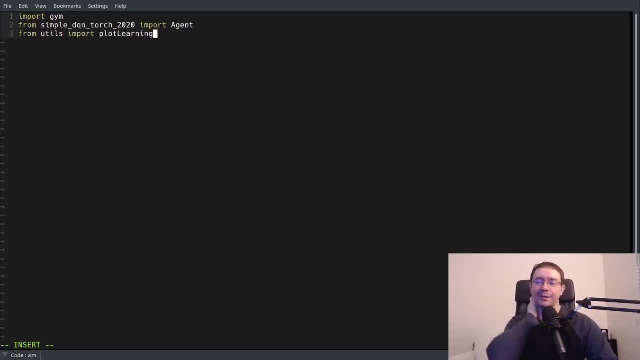 certainly going to get me in trouble because of my incessant renaming of this function. uh, we'll see what happens. it'll be different on the GitHub. in fact, I'm almost certain in this directory that is the wrong name: plot learning curve. we'll do that, just keep in mind, if you're. 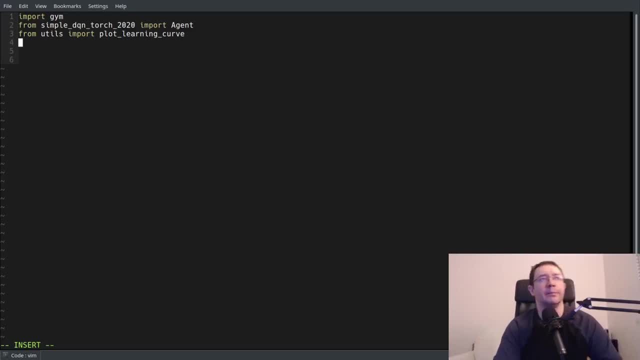 doing a git pull. it's plot learning and I'll. I'll have it correct in the GitHub, but if you're following along you may have a slight difference there. so our main loop is pretty straightforward. the first thing we want to do is make our environment shipmake. lunar lander v2. we need our agent and with the gamma of 0.99, an epsilon that starts out. 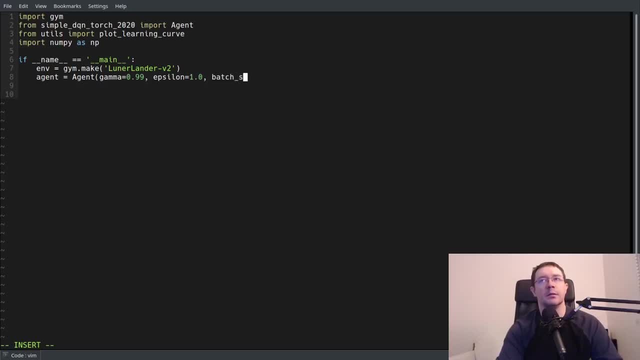 at 1.0, so the agent takes fully random actions at the beginning. a batch size of 64.. number of actions is four. Epson equals 0.01, input dims equals eight and the learning rate of 0.003. we also need a couple lists to keep track of our. 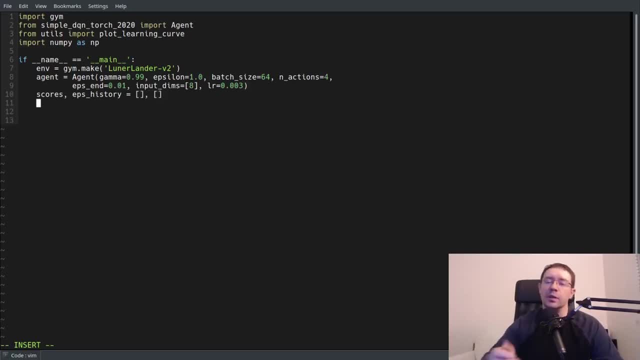 agent's scores as well as the history of Epsilon so that we can plot the scores over time versus the decay in Epsilon over time. and we'll play for 500 games. so at the top of each game we want to reset our score, our done flag. 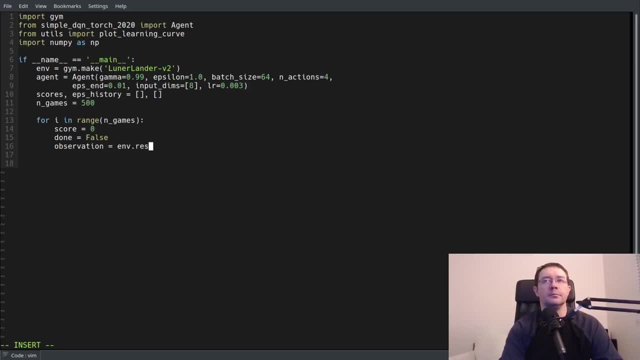 our environment and we want to play each game, and the first thing we want to do is choose an action based on the current state of the environment. then we want to take that action, get the new observation reward done, flag and debug info from the environment. we want to increment the score. 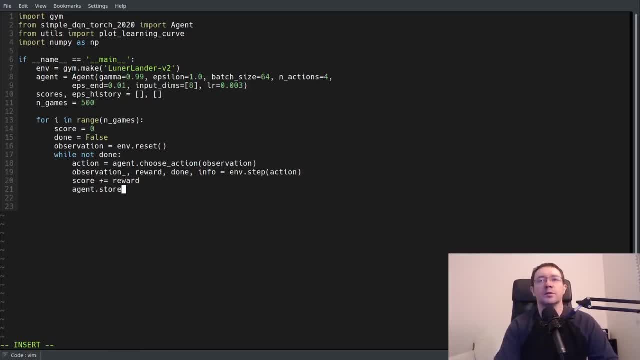 for the episode by reward. we want to store that transition, observation, action, reward and done. store all of those, go ahead and call our learn, function and- very important- set the current state to the new state. i forgot this and it took me forever to find it. i was. 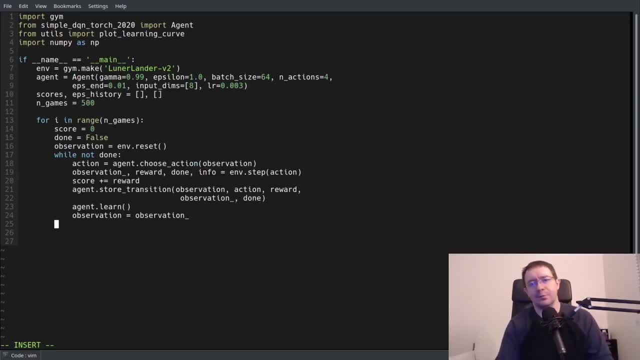 debugging the deep neural network. i was scratching my head, you. you really need that line, otherwise it does not really work. at the end of each episode you want to append the score and the epsilon at the end of the episode. epsilon, let's say average score, equals mpmean scores. last 100 games. this is just. this is just. 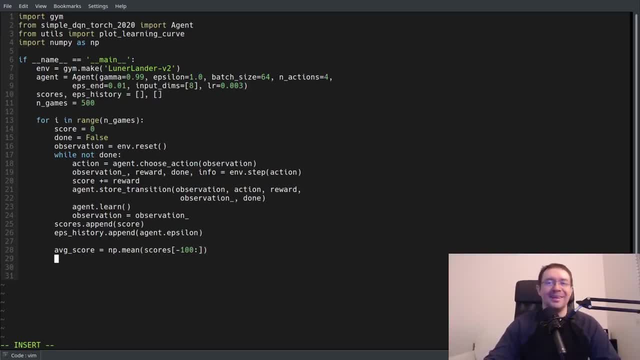 to get an idea of. is our children, is our agent learning, uh, so we're going to take the average with these 100 games, uh, and then we're going to just print some simple information to the terminal so we know that it's running the score, the average score and the epsilon. 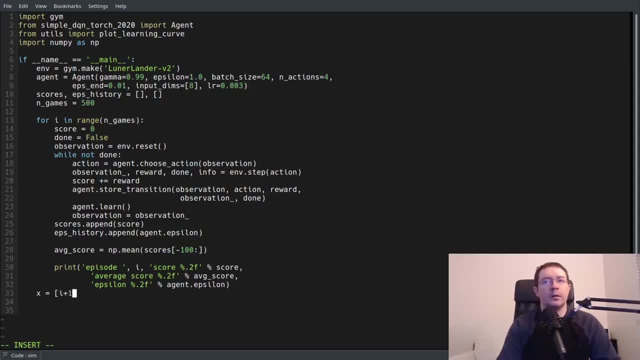 at the end of all, we're going to want to go ahead and plot our learning curve and this is just the x-axis, a file name, our x-axis, the scores, the epsilon history and file name. and if you're new to the channel, uh, just do a clone of my github repo. it may be called, uh, it may be called plot learning curve. 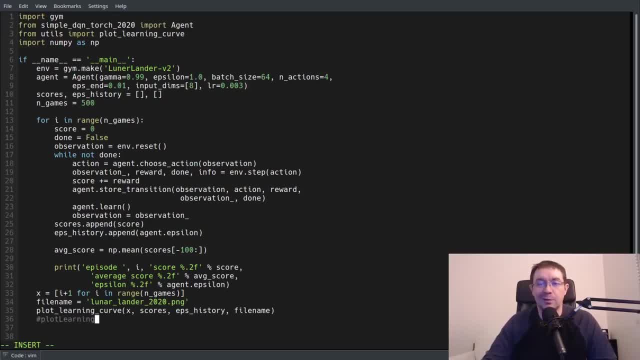 if you're new to the channel, you may want to go ahead and do a clone of my github repo, and then you can do a clone of my github repo. if you're new to the channel, you may want to do a clone of my github repo. if you're new to the channel, you may want to do a clone of my github repo. 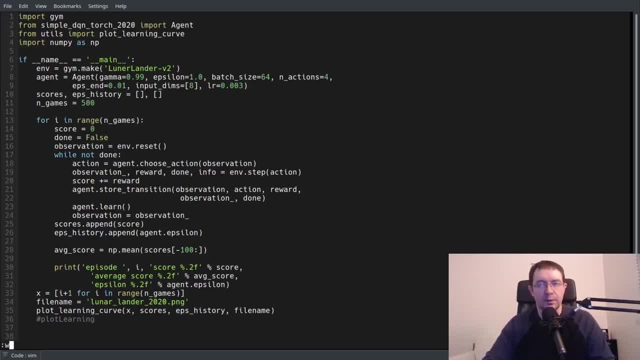 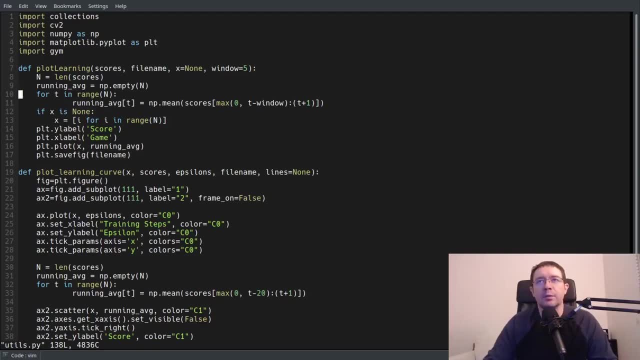 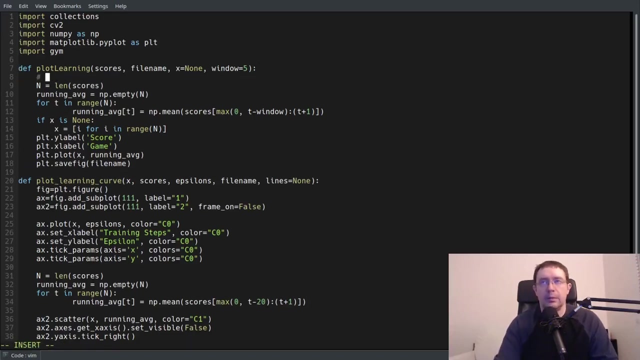 uh, just keep that in mind. so let's do a right quit. and uh, let's check out the utilspy. no, it is plot learning here. okay, uh, scores x, i see. so, uh, this, the, this version, is for boo buddy, this is for um policy gradients algorithms, and i know that because 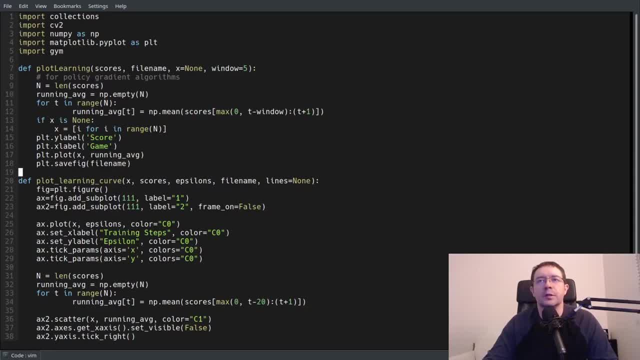 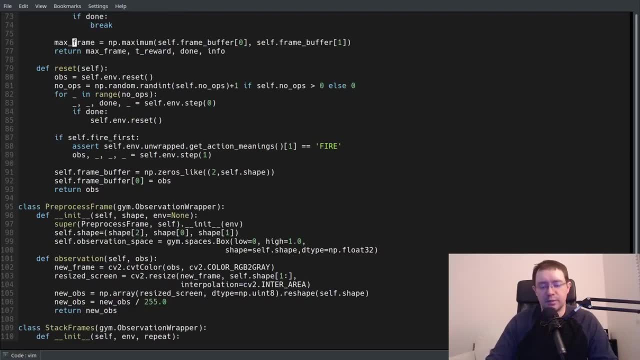 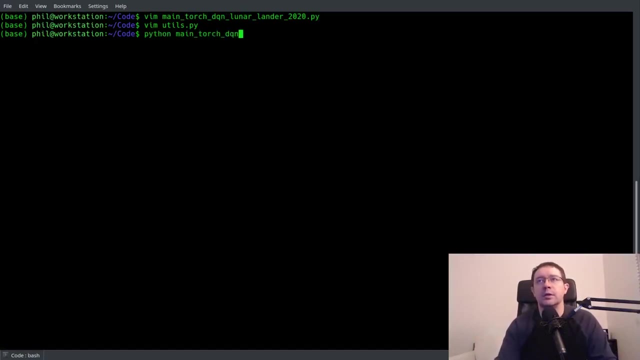 there is no epsilons, so this one here, plot learning curve, is for the epsilons, and i also have a bunch of other stuff for- uh, you know, pre-processing frames and stuff from the course. all right, so let's go ahead and try to run that main torch dqn lander 2020. see how many typos. 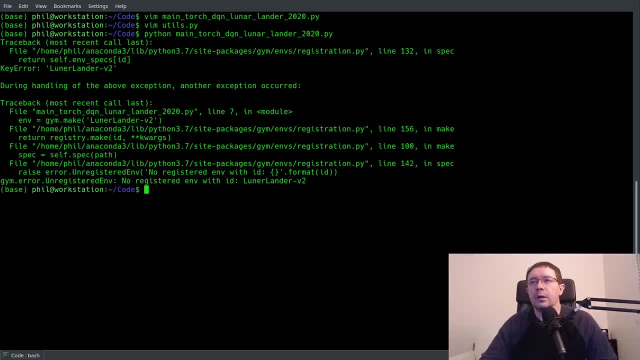 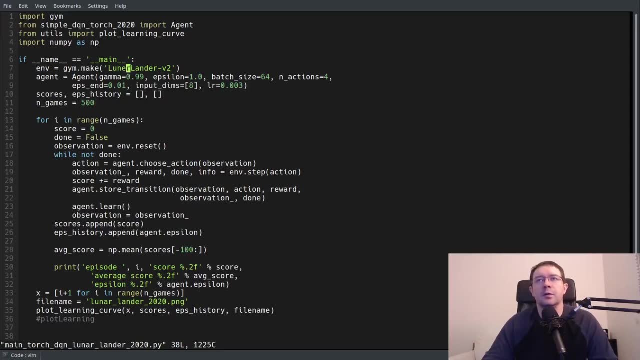 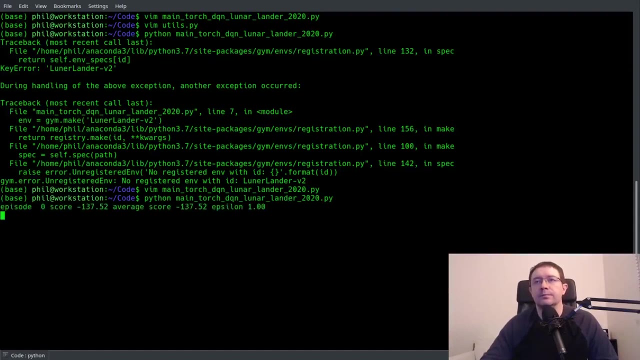 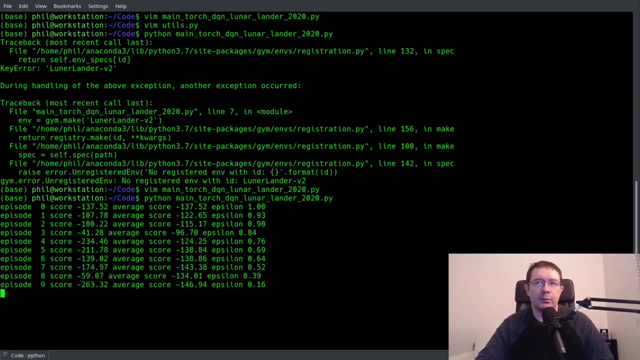 i made: uh, lunaire, oh, that is a problem, lunaire, that is an easy one to fix, easy, easy typo, and that's incredible. there was only one typo. so i'm gonna go ahead and let that run for 500 games and then we're going to come back and check out the results. 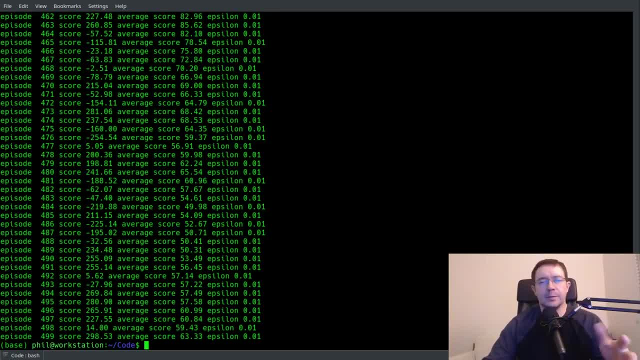 and we are back now. i didn't time this. i kind of wandered off to play with my kid for a little bit, uh, but you can see that the uh performance is a little erratic here now. i believe the reason behind this is twofold. uh, first and foremost, i think, the learning rate of zero. 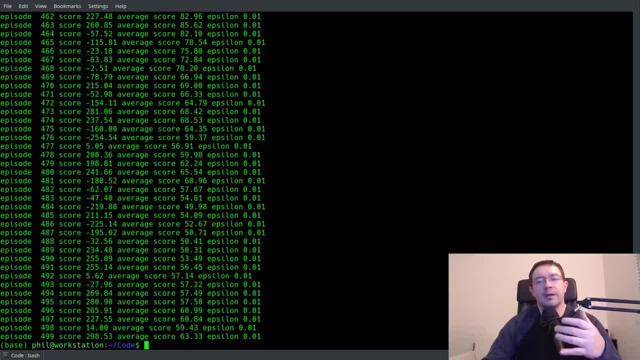 zero three is a little bit too high. so i would recommend that when you play this for yourself, you go ahead and lower that as well. and the second reason is that we do not have a target network, so it does learn. so let's check out the learning plot here. you can see that the agent's performance 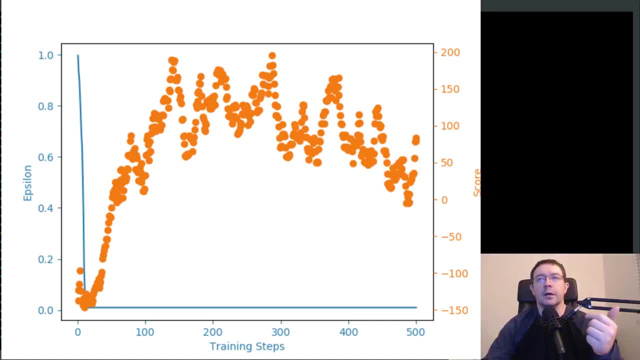 overall increases over time and around um like 250 to 300 games or so, it reaches an average score of about 200, which is considered solved. so it does solve the environment, but then, due to the fact the learning rate is a little bit high, uh, the performance starts to degrade over time, meaning, 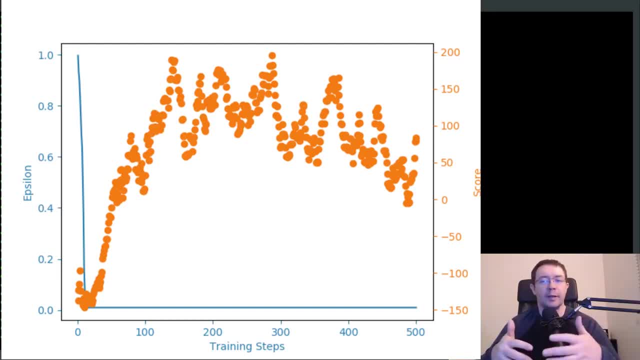 that the agent uh is kind of wandering off from that local minimum where it has achieved relatively good performance. Other thing of note is the oscillations in the performance. This is due to the lack of a target network. So a target network tends to help with model stability over time. 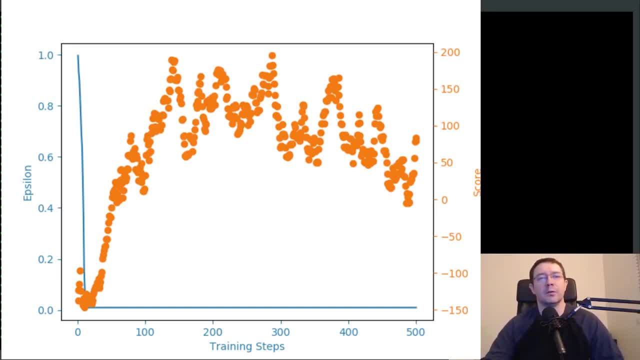 But in this case it doesn't seem to be a huge, super big deal. So that is the agent's performance in a nutshell, minus some tweaking. 003 is a little bit too high. When you go ahead and run it for yourself, use 001 or something a little bit lower. 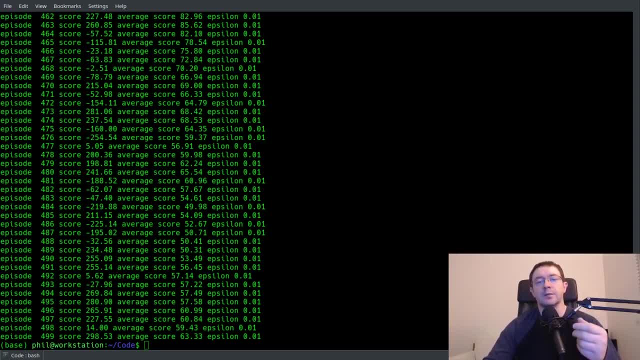 and you'll get better performance. So everything else, conceptually, is the same. You don't have to tweak anything other than learning rates, maybe some model parameters such as the number of neurons in the hidden layers, but that's up to you. That is how you do deep Q learning from scratch in the simplest possible case. 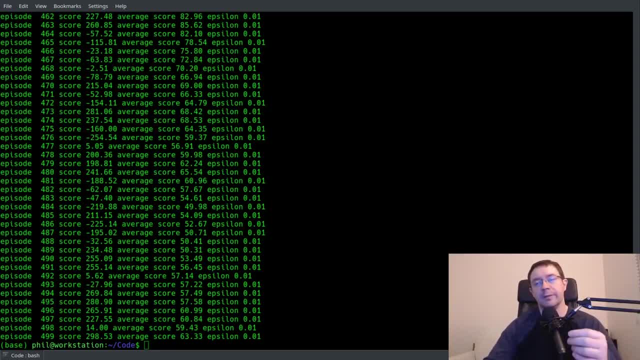 That is, a deep Q learning agent with just a replay memory, no target network, And this can be employed in a wide range of very simple one-dimensional environments, meaning you don't input a matrix, you just input a single vector, And so I hope this has been helpful. 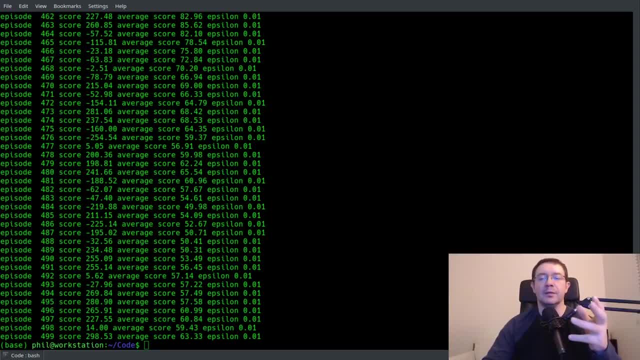 Any questions, comments, leave them down below. I'll try to get them to them. I have been getting inundated with questions and comments lately, so my ability to answer is compromised, but I will do my best nonetheless. If you've made it this far, please consider subscribing. 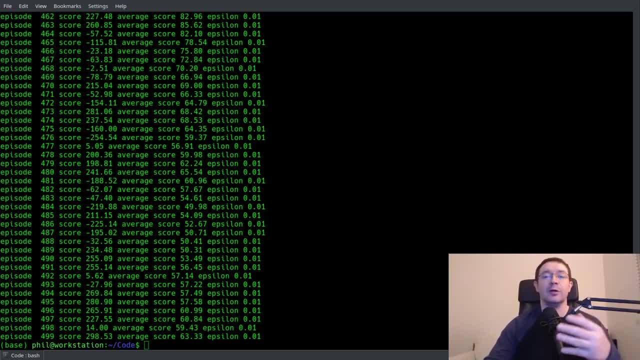 And don't forget my new course, Deep Q- Learning from Paper to Code, where you learn the how and the why of all this stuff, as well as how to turn deep reinforcement learning papers into code, is currently on sale for the remainder of the month of March.